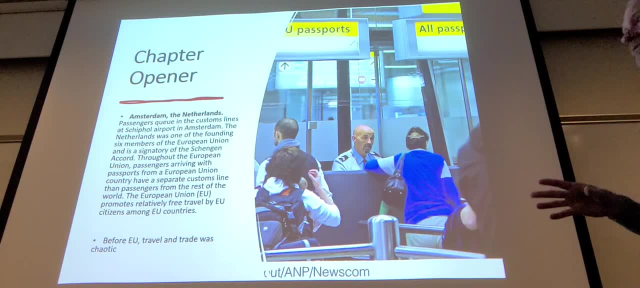 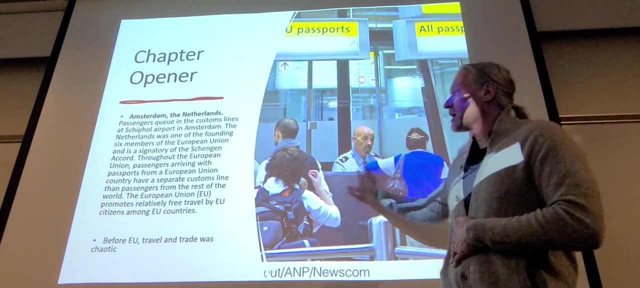 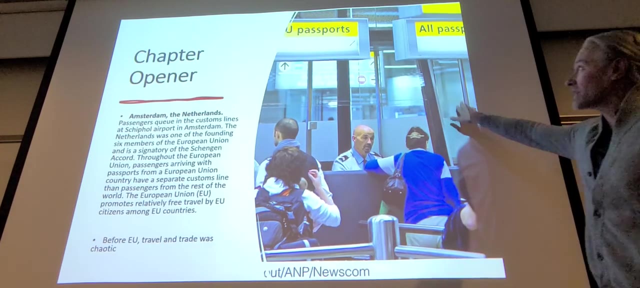 tracing information, Just kind of Again and again and again. So not the most fun, but it was still good to travel. These lines were really long this year. I would say there was one time in Portugal. was that these exact lines, with these exact? 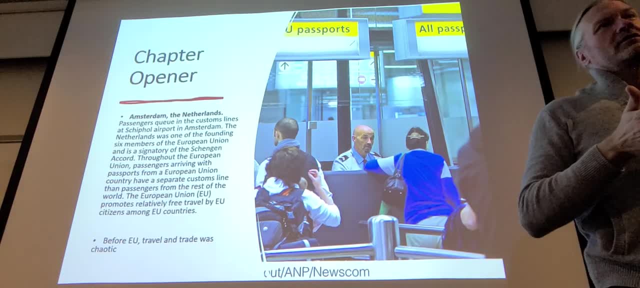 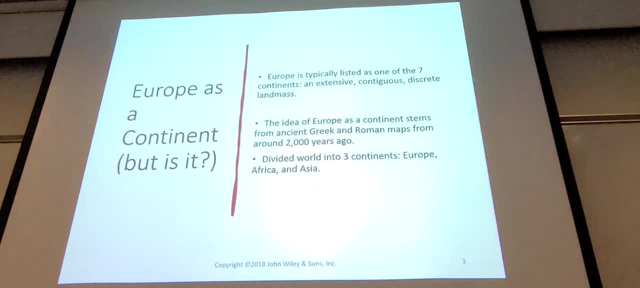 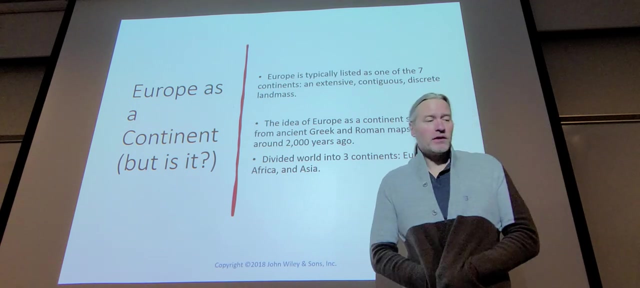 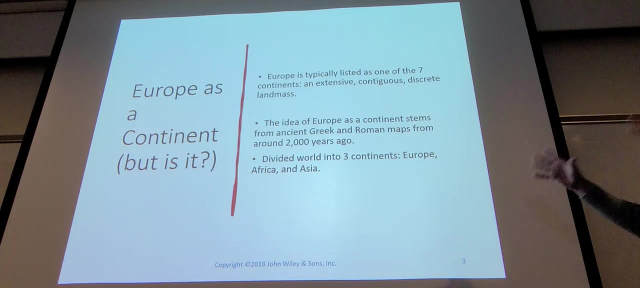 names stood in place for three hours without moving, So it was a little something So jumping off into our reading. Europe, Right, Usually a place that people think of as its own continent, even though, from a geographical perspective, well, you have Eurasia as a continent, right. 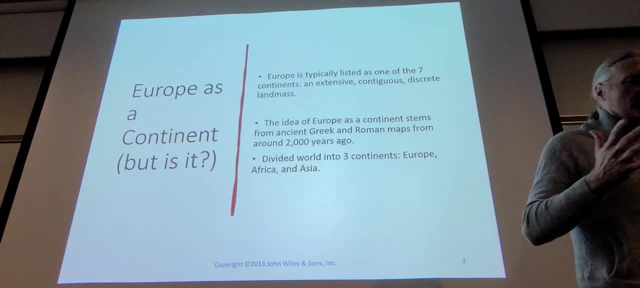 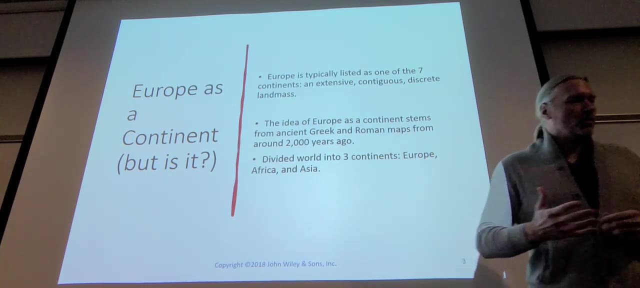 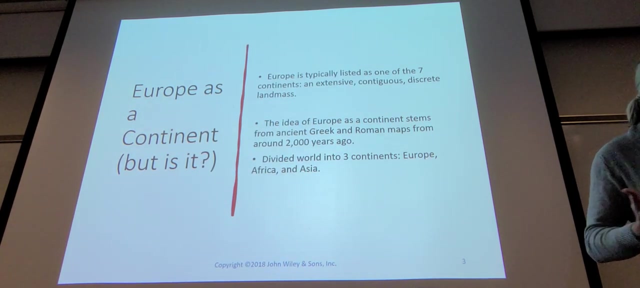 Europe isn't actually distinctly cut off from the rest of your Asia, Although, in the kind of mindset that European set up, It was right, wanted to divide the world into these kind of three categories, just as a simple way of thinking about the world, but also, strangely enough, well it lined. 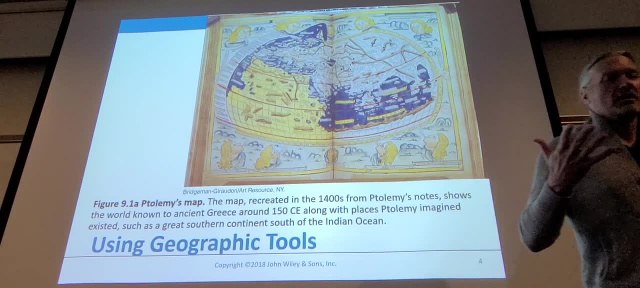 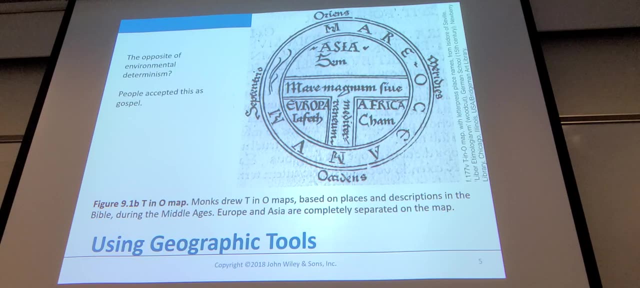 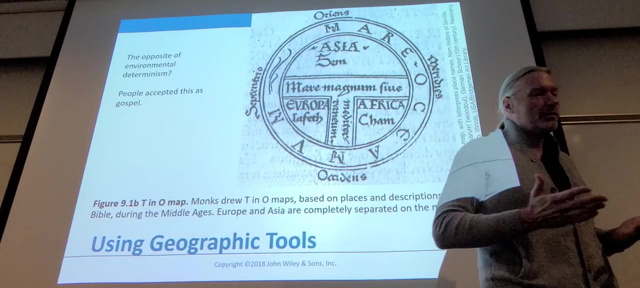 up with Europeans conception of the world, specifically in a number of different ways. one putting themselves on top also, if you remember from the readings, trying for, for whatever reason to say, the world was in the shape of a cross. a lot of well Roman Catholicism was was the rule of the day in the Middle. 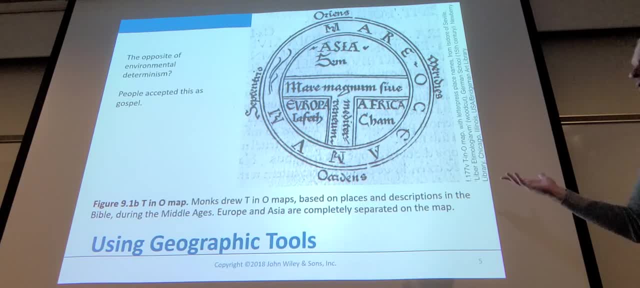 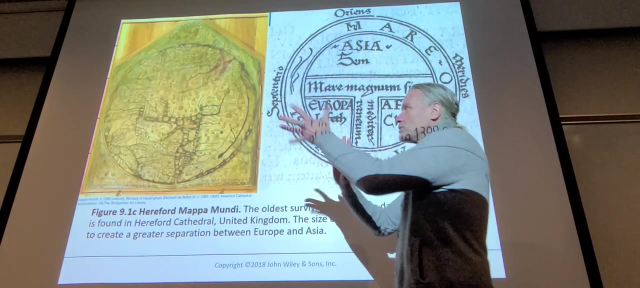 Ages and a lot of people in Europe took such things like a map like this that doesn't really make a lot of sense, but took it as gospel reality, right even to the point. when making actual maps of the region, they would try to try to squish things around as much as possible, even as new. 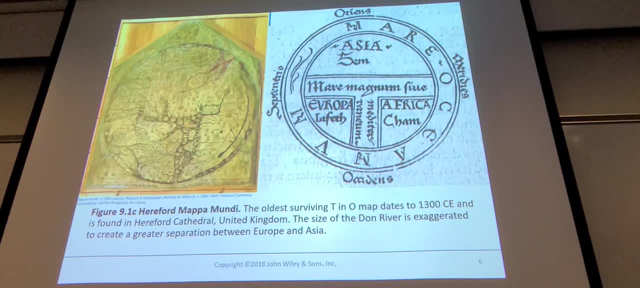 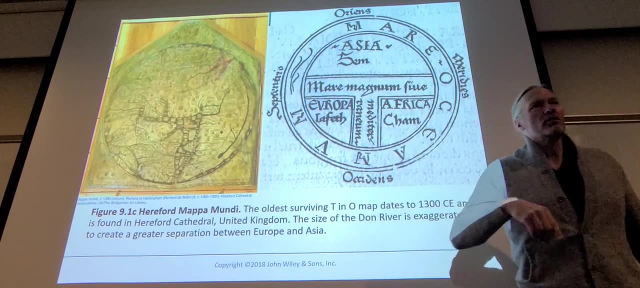 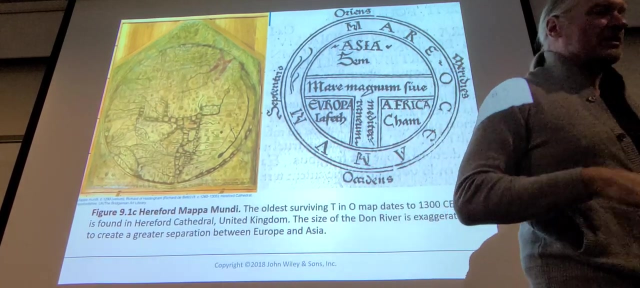 information was coming about the shape of the world. so, for example, you know, there's not an actual circular ocean that surrounds this whole area. right, it's like it's around Earth, but there isn't an endless ocean. so it's one of those weird things of history that still kind of has a legacy and that Europe is. 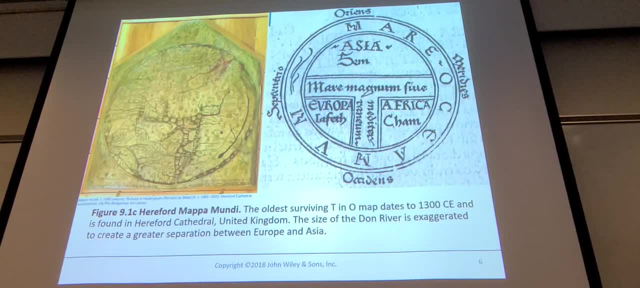 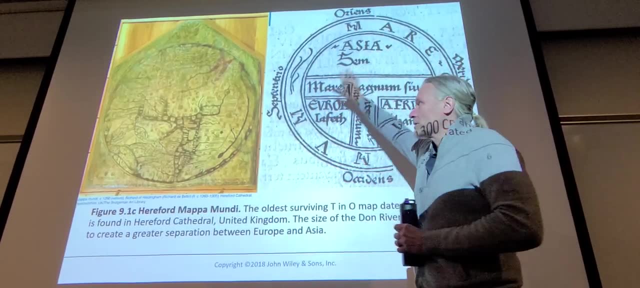 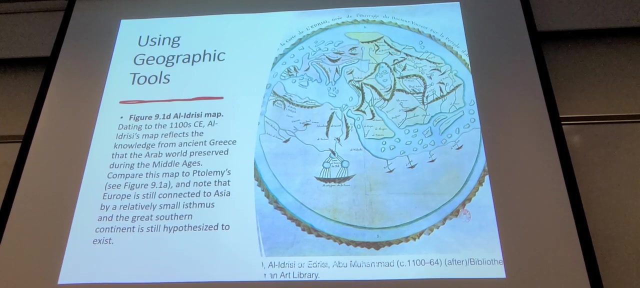 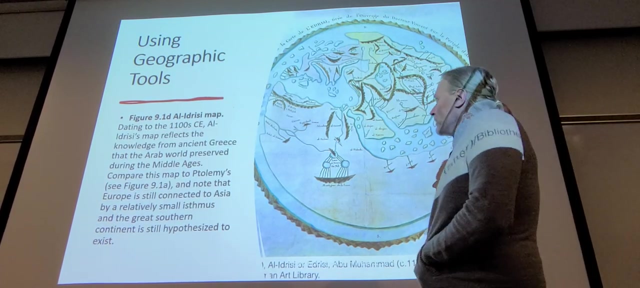 still often thought of as a it's own continent that is separate from the rest of the world- right Europe separated from Africa, from Asia, but it's actually completely connected to Asia through time, as I said, even when new knowledge was coming about how the rest of the world was shaped and things were getting well, more and more information. 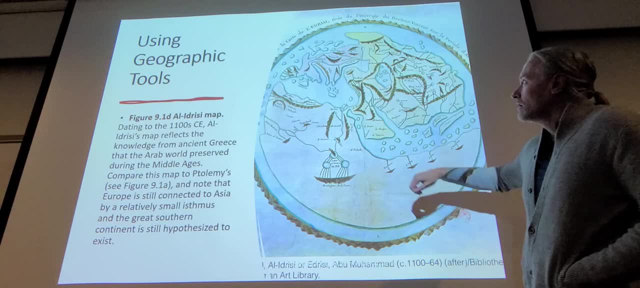 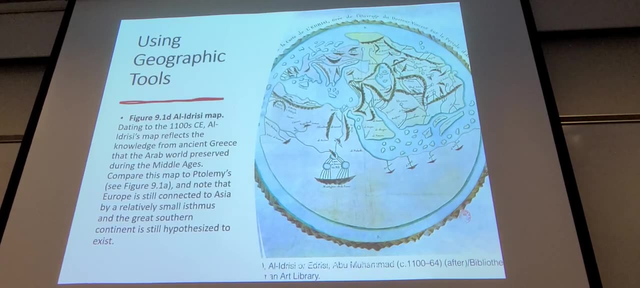 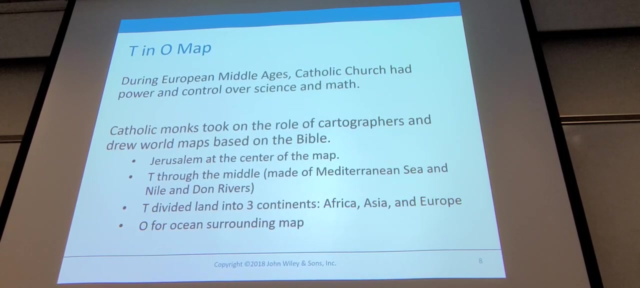 was coming, especially after the Dark Ages, from a lot of centers of knowledge that were in the rest of the world about the shape of the world. Europeans knowledge of that shape of the world starting to devolve, starting to change. as I mentioned, having a TNO on the map was really forced into. 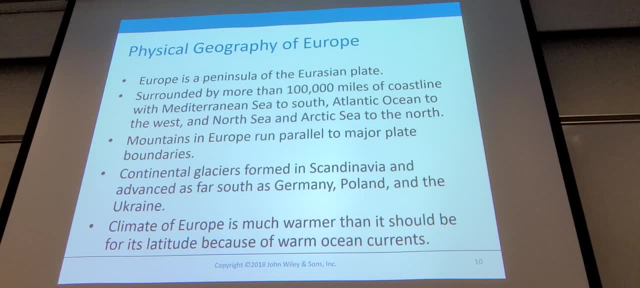 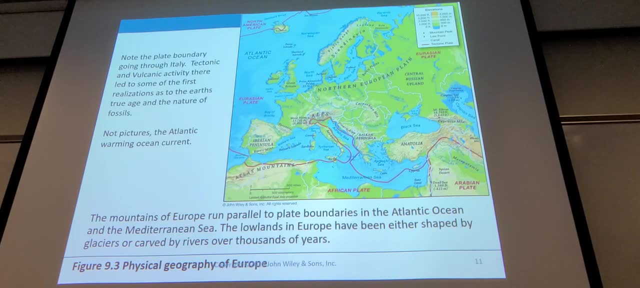 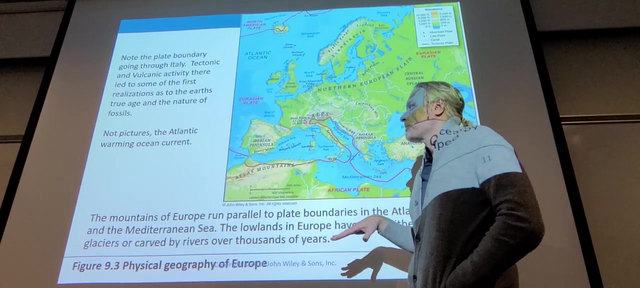 place. physical geography of Europe. let me get to a picture of the actual continent. so, as you can see, the direct origin of Europe was in the most part through the ancient world. see right, very connected to, to, to the rest of the world. let's see here what. 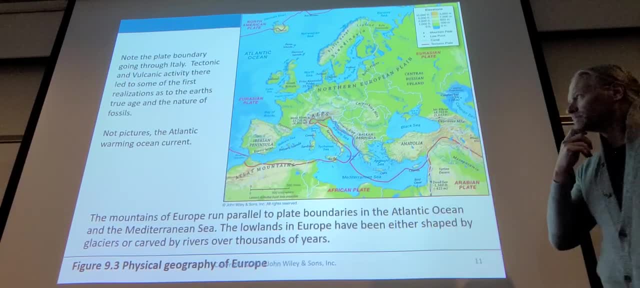 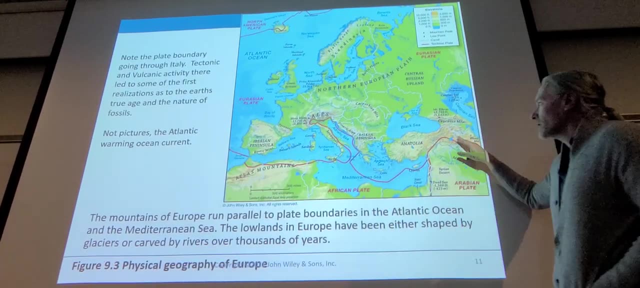 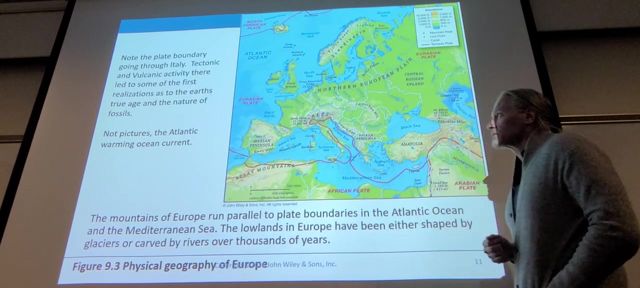 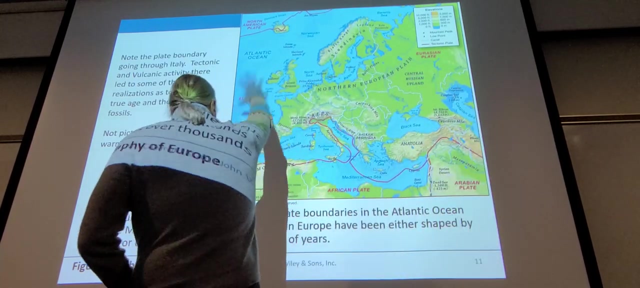 can I say about this? well, note the plate boundary that goes through Italy and also Turkey. this plate boundary, well, like many of these plate boundaries around the world, there's a lot of earthquakes, there's a lot of volcanoes, Europe itself, if it wasn't for the Atlantic drift bringing warm water. 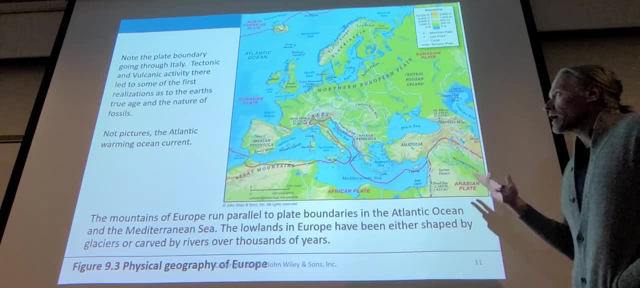 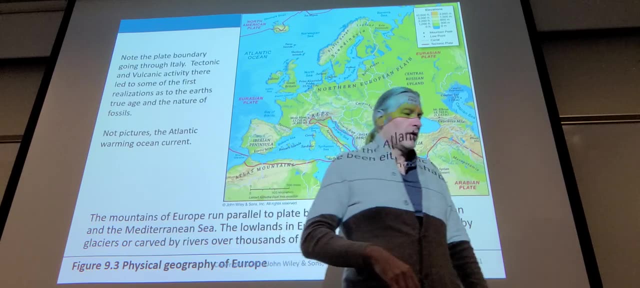 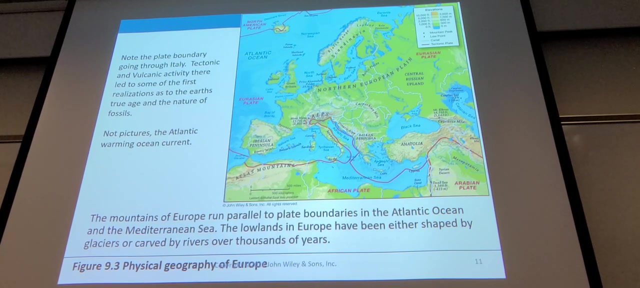 off the, from off the coast of Africa, Europe would actually be much colder than it otherwise is. if you ever look at a globe, for example, line up how far north and south Europe is compared to, say, Minnesota, you'll notice this a lot: the striking difference in temperatures, but also what this is made for the 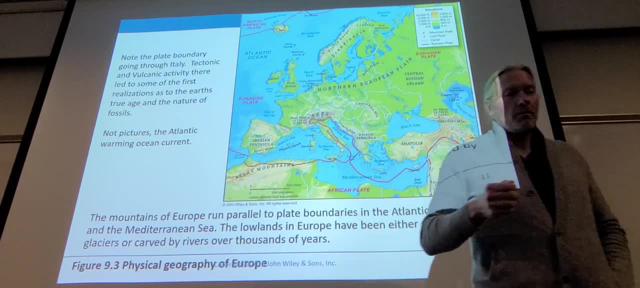 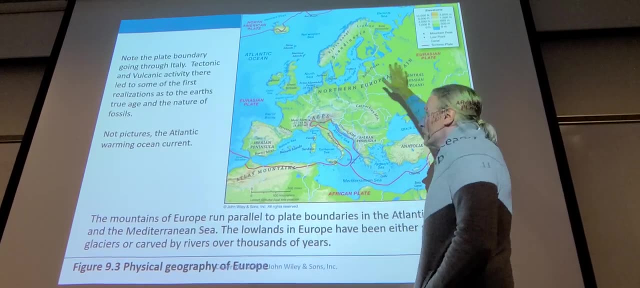 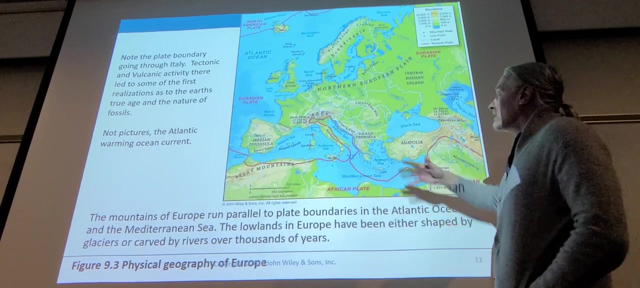 climate of Europe is has made it a much more moderate climate, without a lot of extremes. now, the further into the continent you go, the more extremes you have, and of course, our next chapter is taking us further in. otherwise, I'm sure you notice, this chapter talks a lot about Eastern Europe. and then our next, 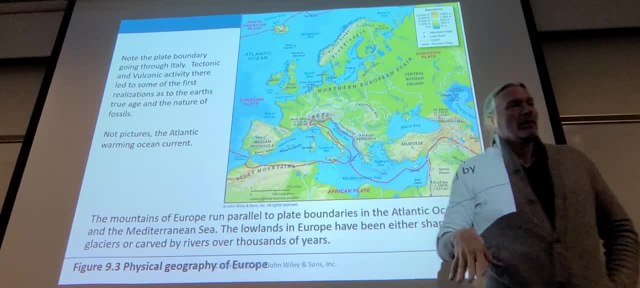 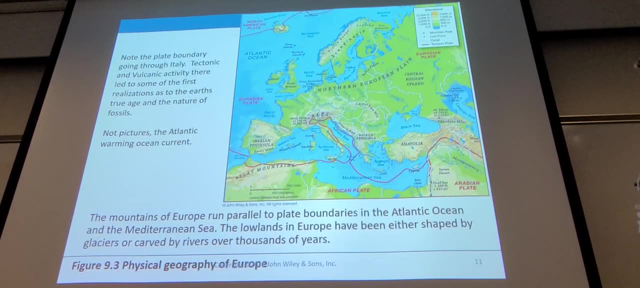 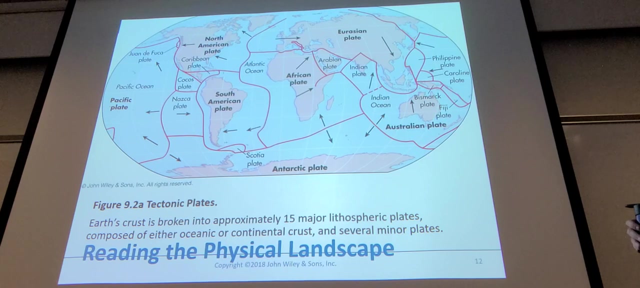 chapter that is supposed to be about Eastern Europe talks a lot about Western Europe, but that just shows you how interconnected the whole area is. uh, let's see what else could I tell you here? that's it about this one: a larger picture of these plate boundaries we've 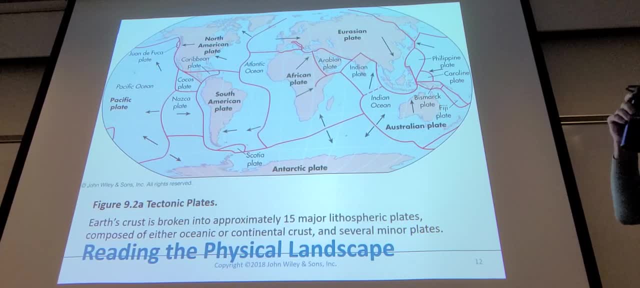 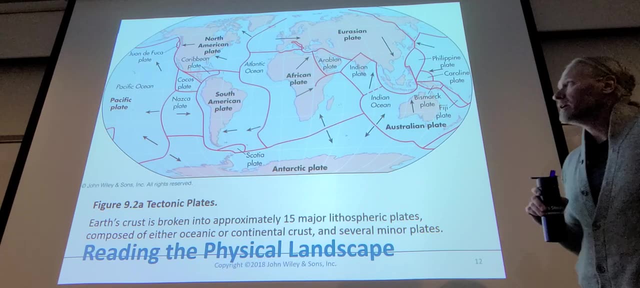 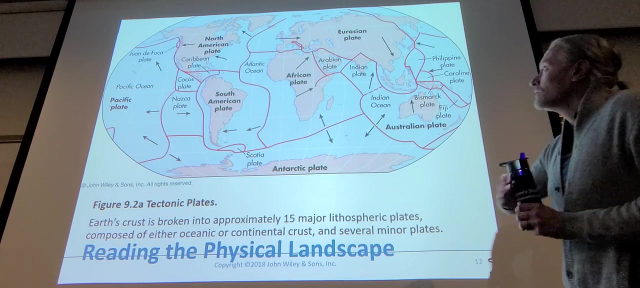 talked about a lot of these, as we have covered the different areas through time. this is yet another example of if we're talking about continents and if we're dividing them up, like using plates and plate tectonics, you still have. you have a Eurasian plate right, not a European plate that's different from an Asian plate. 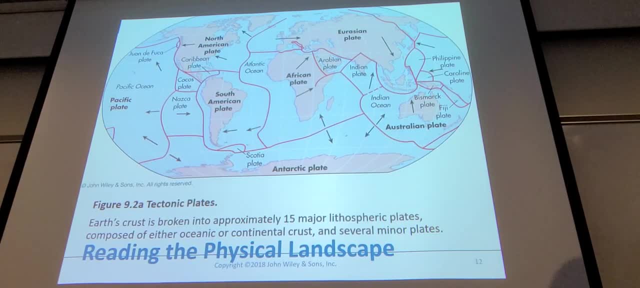 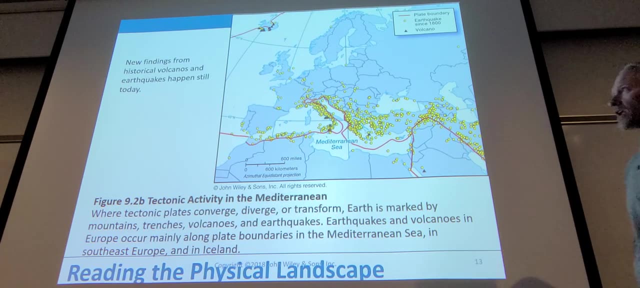 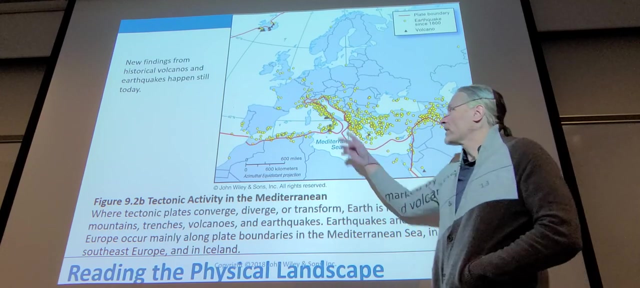 plate. that's different from an Asian plate. that's different from an Asian plate. Eurasian- another map in the book looking at specific tectonic activity. um well, you know, it's actually a lot of this. uh, specifically the volcanoes in Italy. that led a lot of people to. 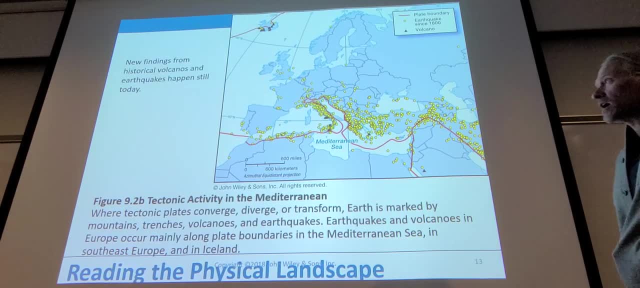 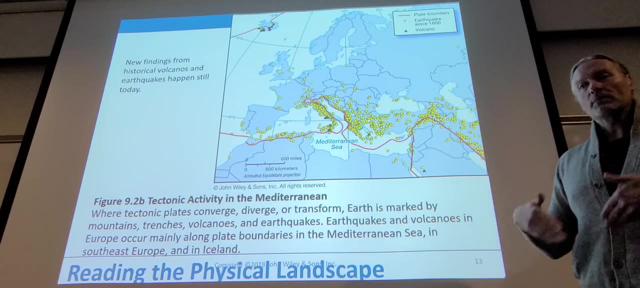 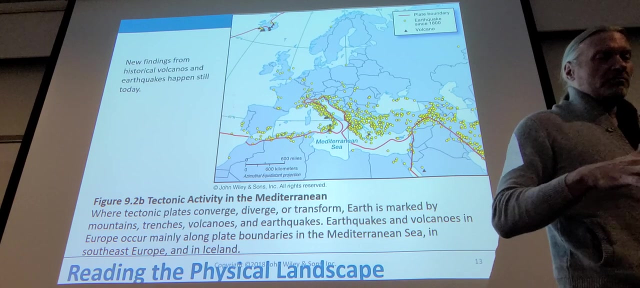 believe well to figure out things like, um, the the age of the Earth, right? um, because, well, Mount Etna, I've been putting out a steady amount of lava throughout the years, and a number of scholars while they, they added up like, well, Mount Etna puts. 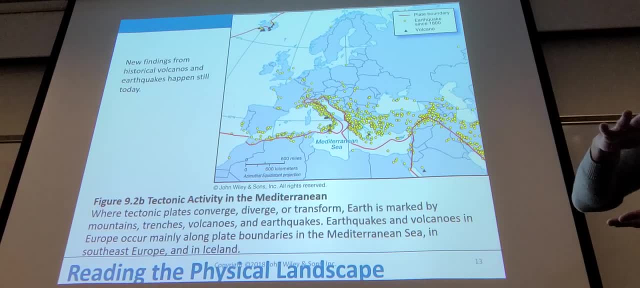 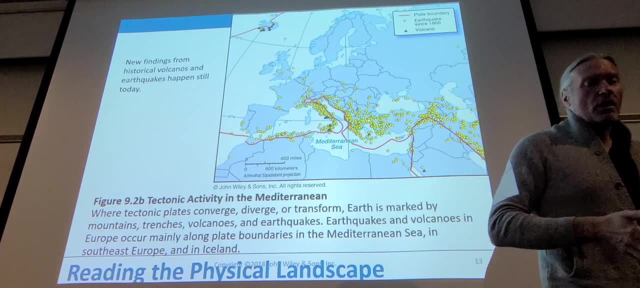 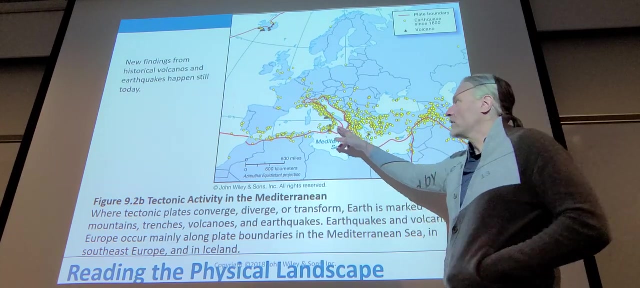 out this much volcanic, uh lava per year, and then you add up how big the mountain is, um, and then, what is more, looking under areas of the mountain and finding fossils. you can then date those fossils right, uh, and so a lot of the fact that this is along this boundary helped with that. 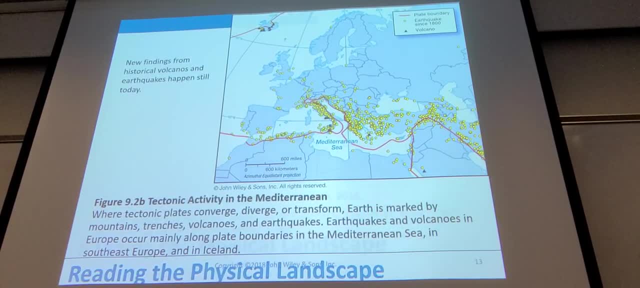 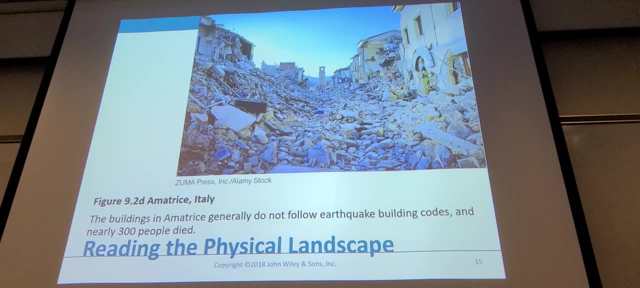 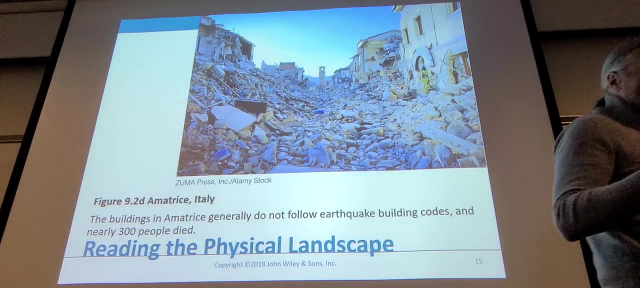 kind of knowledge, um, so it's not just a destructive force, um, although it is obviously a very actually destructive force, similar to other areas of the world that we looked at. when it comes to damage from earthquakes, very often places that have um kind of new building codes uh, tend to have less. 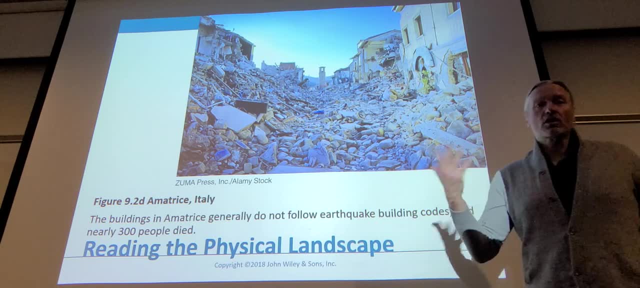 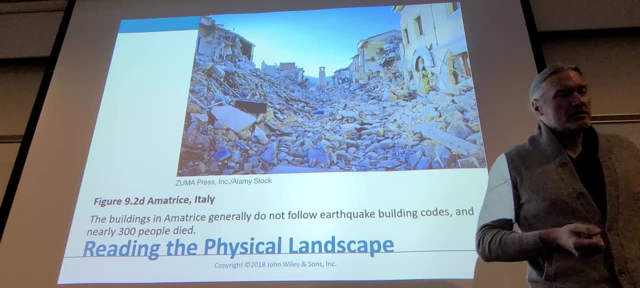 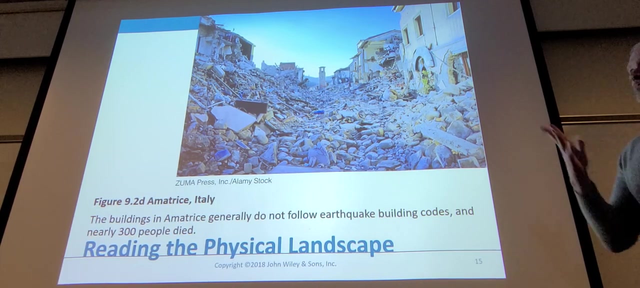 damage, less deaths, but, of course, less places that have historical buildings. of course, when those buildings were put in, there weren't such things as building codes. a lot of historical places can have lots of ruins. um, and you know, in Italy, every year or two you'll you'll see some often gorgeous old buildings that have been destroyed from earthquakes. still happens. 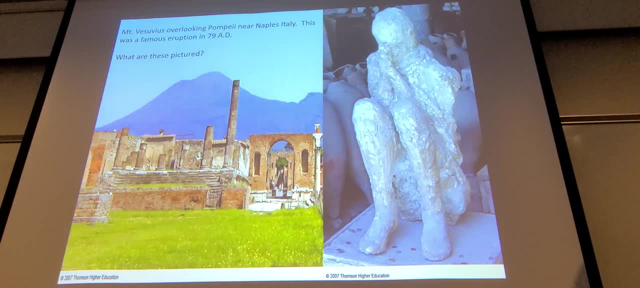 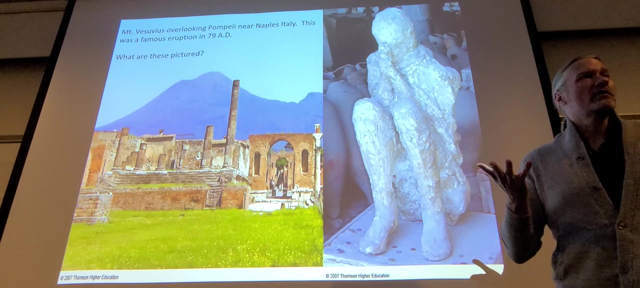 all the time. uh, Pompeii, kind of one of the most famous um volcanic eruptions. uh, again in Italy. um, not that many students this year have traveled that much. I suppose it's probably due to the pandemic. people maybe have read about Pompeii, um, maybe you've seen depictions of little figures. 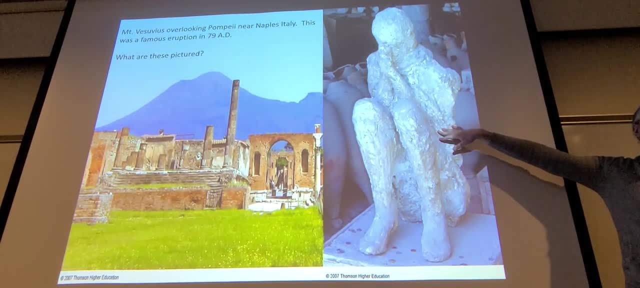 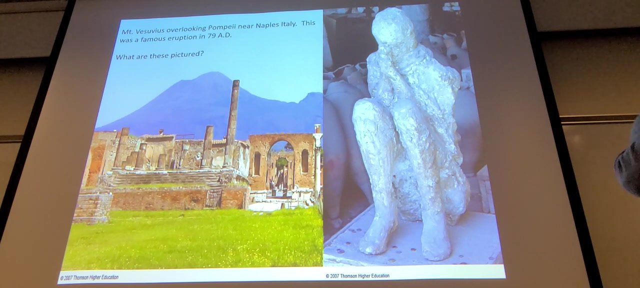 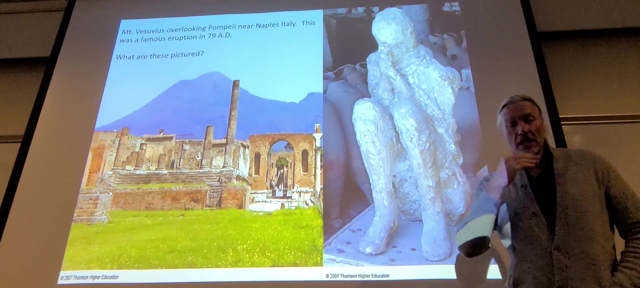 like this when it comes to volcanoes. uh, is this familiar to anybody? like if you're reading a news article about volcanoes, do you know what this is? that's the. so Mount Vesuvius, Mount Vesuvius, yes. um, it could have also been trying to breathe, maybe. uh, it's it. it's interesting because, well as 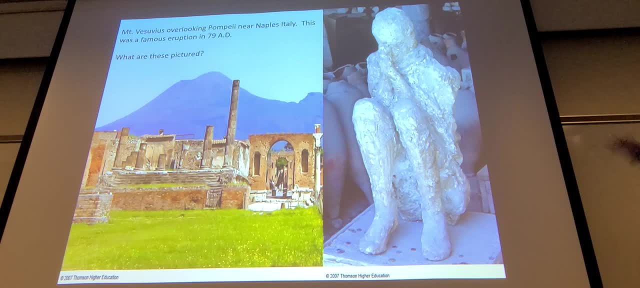 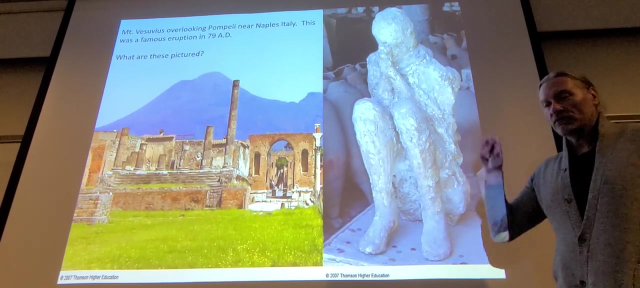 you say, um, there were different types of eruptions and different kind of things that happened, uh, and you know there's still. like Pompeii was on the news just this week because they found, um, what had been a slave quarters. um, well, what this is, you know, if you have a lot of volcanic ash covering up, 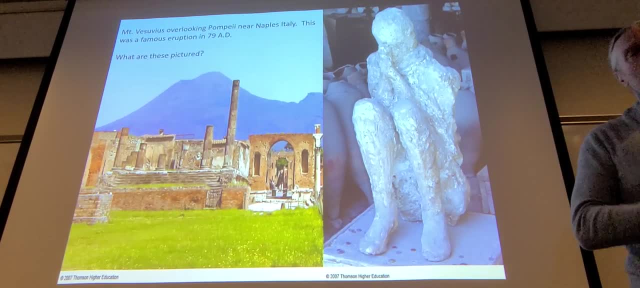 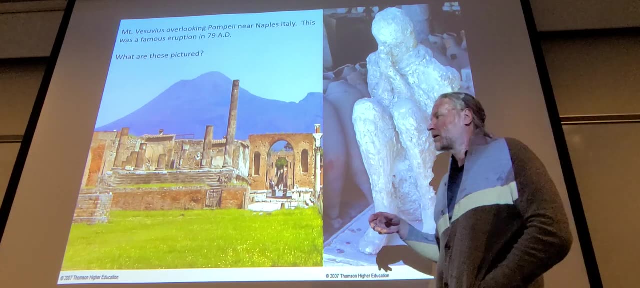 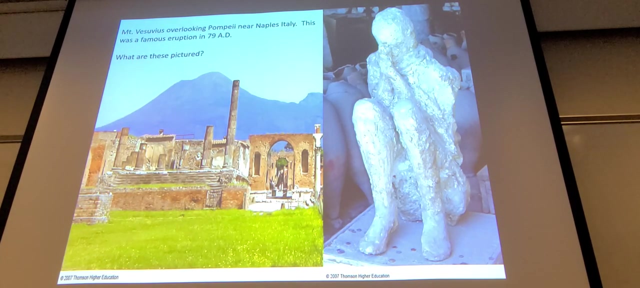 um, well, let's back up when they first started kind of digging up this area and trying to figure out what it is. there had been stories written about volcanic eruption and whatnot. um, and when people were digging, well, obviously sometimes you find skeletons and stuff right, sometimes you find just these empty spaces, that there's nothing in them. uh, and people hypothesized. 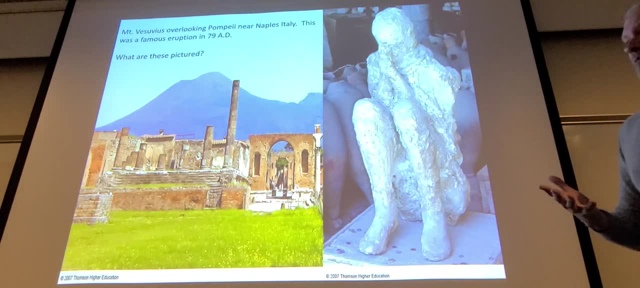 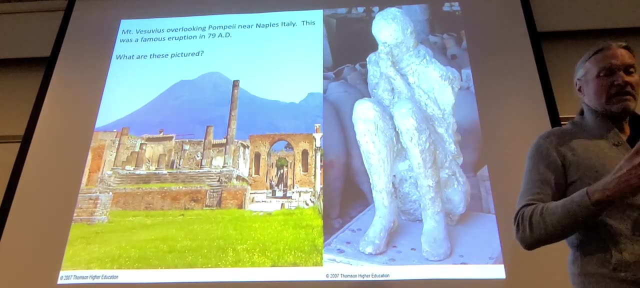 through time that it was possible that, um, if organic material was covered in this ash, um it could be just completely desiccated and waste away and it would just leave these kind of empty pockets. and so what they did was, when they were kind of excavating, if they did find. 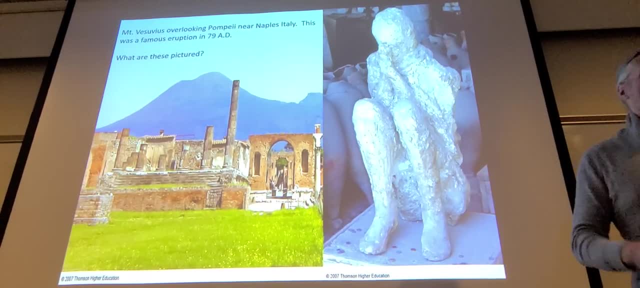 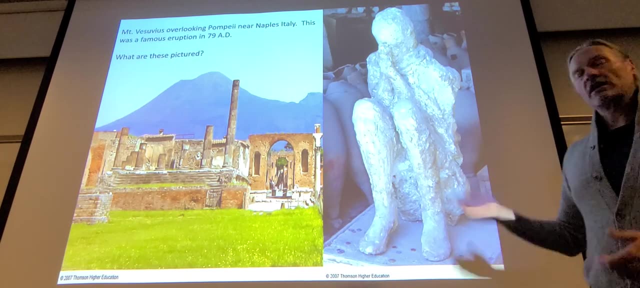 one of these empty pockets, they would fill it full of plaster right, dump a bunch of plaster in there, let it settle and then you take it out just to see what shape it is, and sometimes it's like a horse and different organic things. but sometimes you know, people are organic things as well. 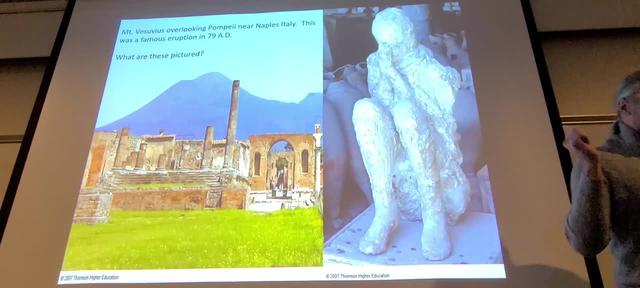 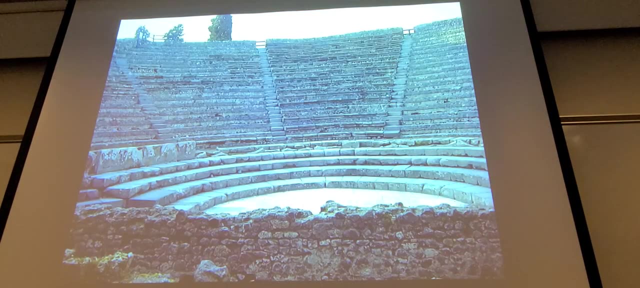 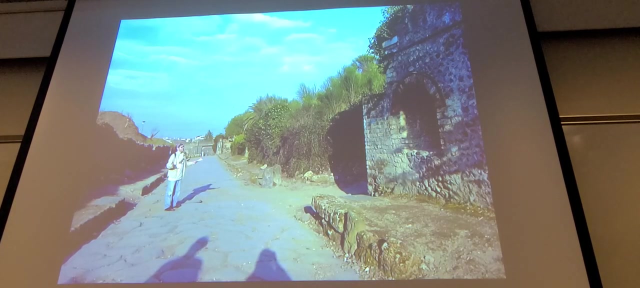 um, and so that's that's what these are about. um, and, like I said, they're still finding these today. um, like, like just last week- uh, this isn't from the news, though- this is when I went, uh, in college. uh, this is old. um, one of the interesting things about Pompeii is it was a, for the time, very modern city. this: 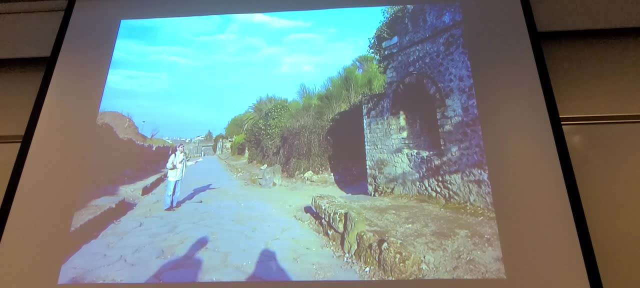 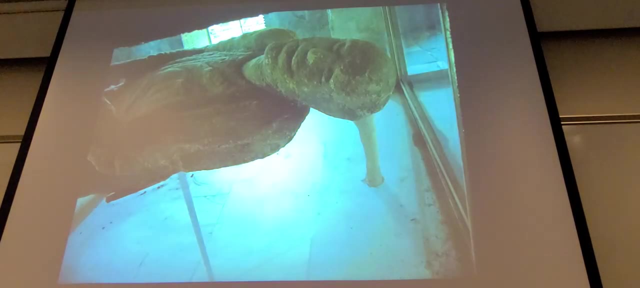 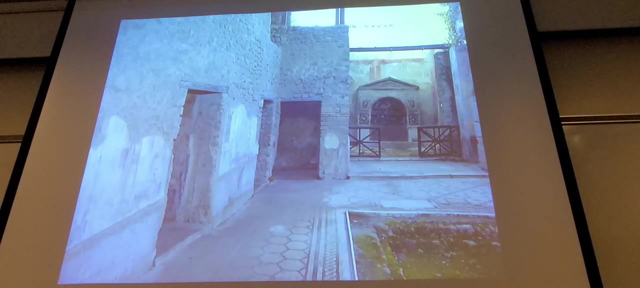 is just streets, um, and these are all had to be excavated. these were all under a lot of volcanic ash, not lava, because, as you can imagine, a lot would be much more difficult to excavate through. um, there's lots of these little figures. oh, it's a little dark. I have a question. yeah, 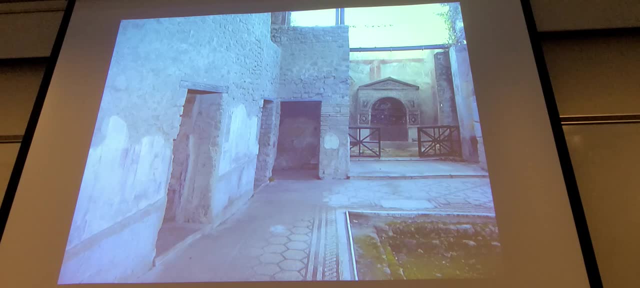 a couple different reasons um, one being actually areas where tectonic plates come together often have really valuable metals, because the metals are heated up and they kind of leak through and so there's lots of money to be made. um, and also there's just a thing happens where people don't think something's gonna happen to them, right. 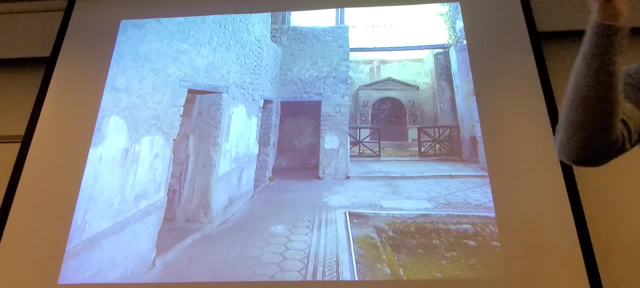 they think something's gonna happen to everybody else but won't happen to them, right, it's like, oh, this thing we're talking about it's not going to happen in my city, right? um, there's that kind of an attitude, and enough time goes by sometimes that they're just minor eruptions that they think. 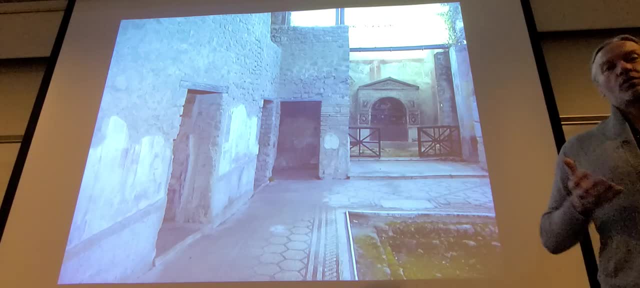 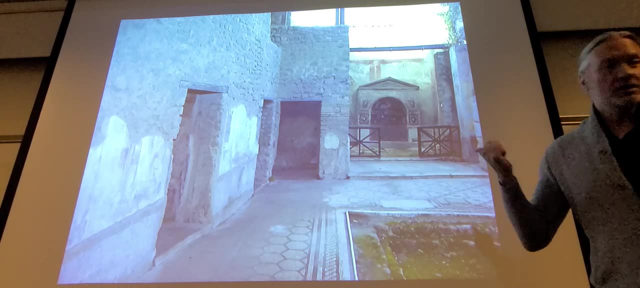 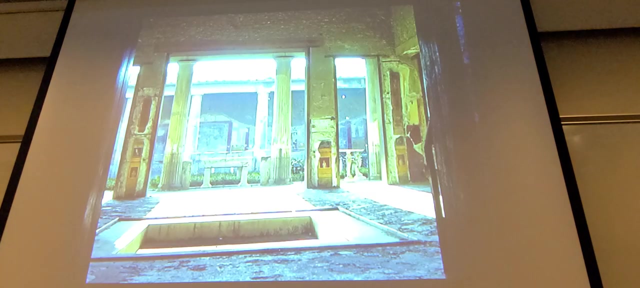 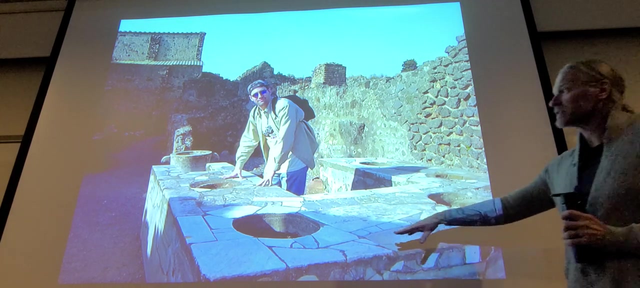 it's not going to be, uh, a gigantic one that kills the whole city. uh, and they would be wrong, right? um, uh, just some more excavated areas, you know, and again, it looks not dissimilar from more modern day homes. um, so, my college roommate, but he's just standing here to give this some scale. this was, uh, the. 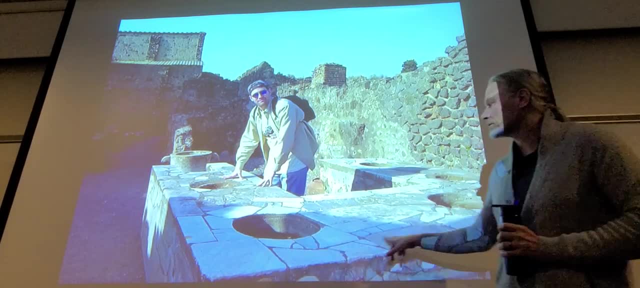 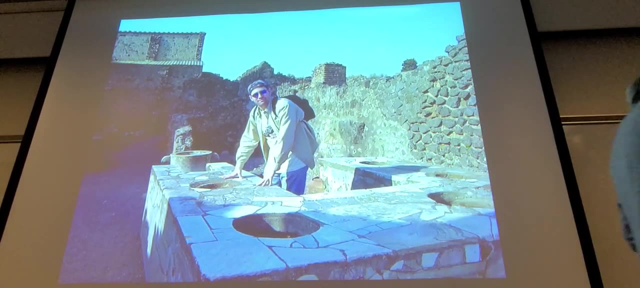 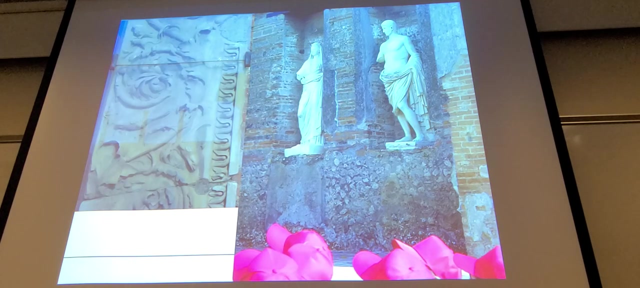 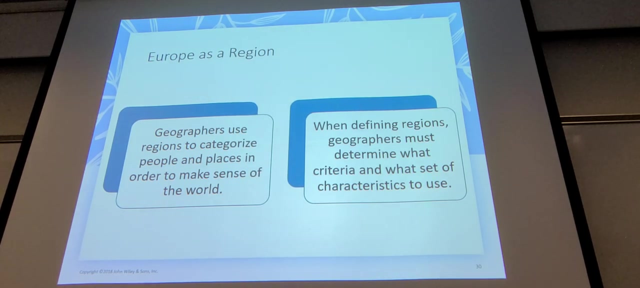 equivalent of fast food at the time. uh, they would have these fires under here, you'd have pots, you'd have some water people. this is a little street here. people would come up and purchase their food. all right, a little bit of Pompeii. um, back to back to geography in this chapter. uh, well, as I said before, and we're talking, 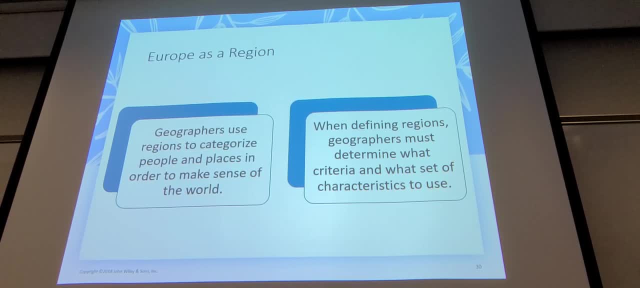 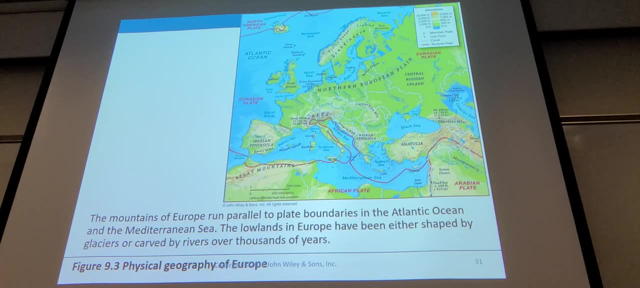 about Europe as a region. um, not as a separate continent, because, again, it's connected, uh, but as a region that makes some distinctive amount of sense. um, right, because culturally, uh, it's well, it's a place that has more interaction, uh, locally, right, um, although there's lots of. 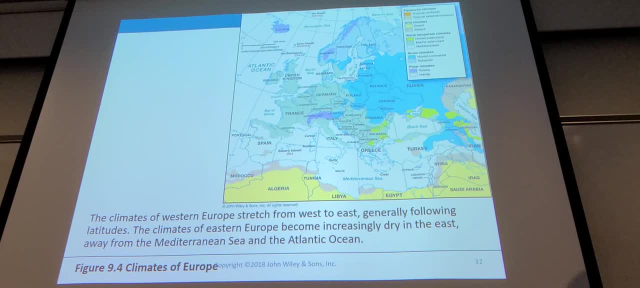 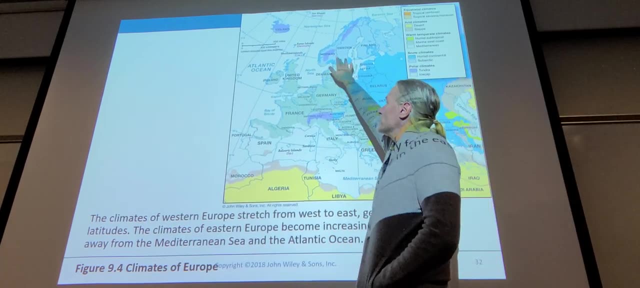 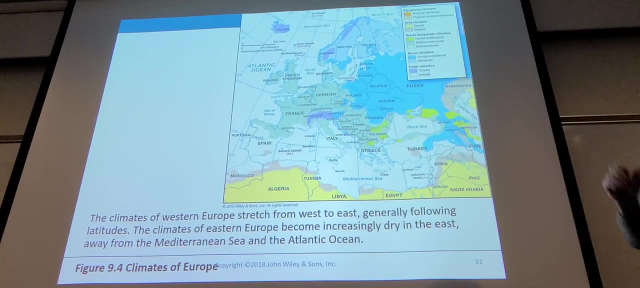 connections with the rest of the world. obviously, uh, I'm mentioning the climate earlier. uh, you can see some areas here that have some polar climates. these are also areas that, when there have been ice ages, this is where the glaciers built up and spilled across from. um, let's see what else can I? 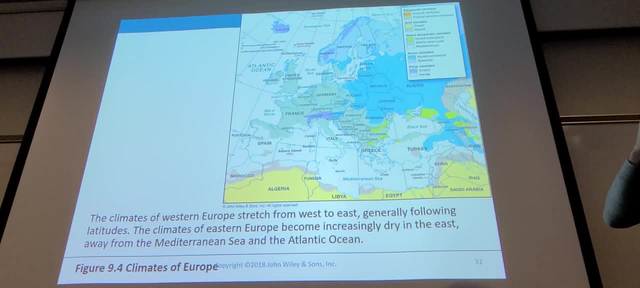 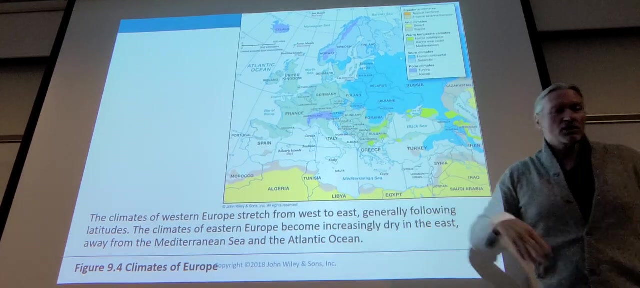 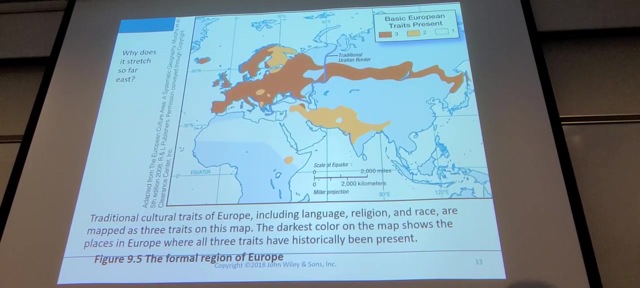 point out from here. um, like I said, the the climates are much more moderated than they would otherwise be because there's so much, you know, water is a very moderating influence. the climate and weather, uh, and this is such a large Peninsula, all right. uh, there's another map from the book looking at, if you're going to try to define Europe. 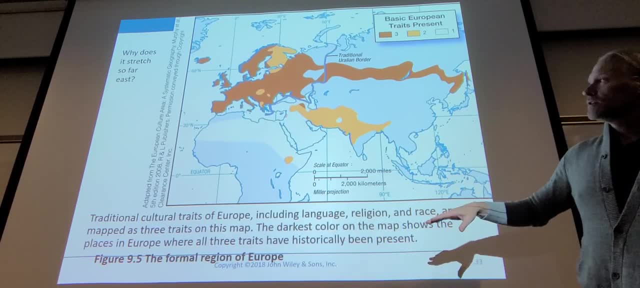 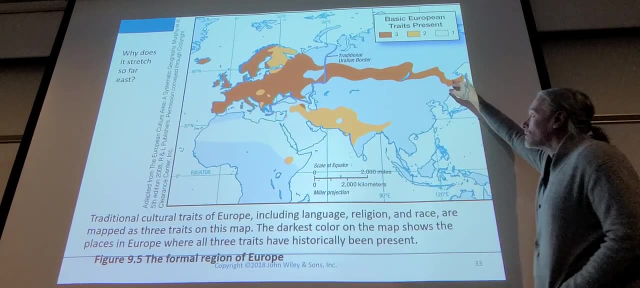 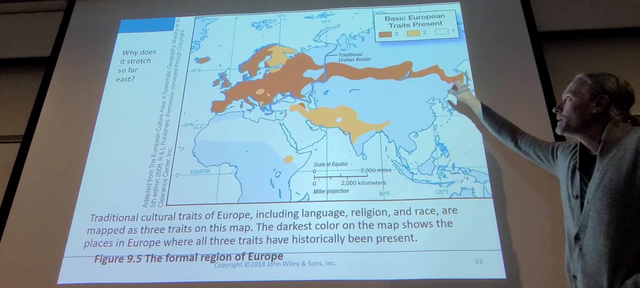 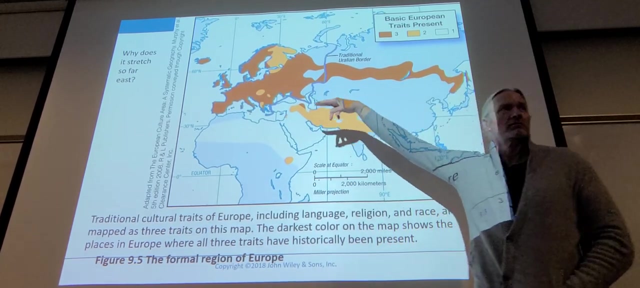 um, looking at the categories of language, religion and race, what would you have? um, well, again, you see, Europe is very connected to all the rest of Asia, right, going all the way to the coast here, and this is Japan, just for reference, right? um, people know why this, this cultural trait, extends right along here. anything else going on in this? 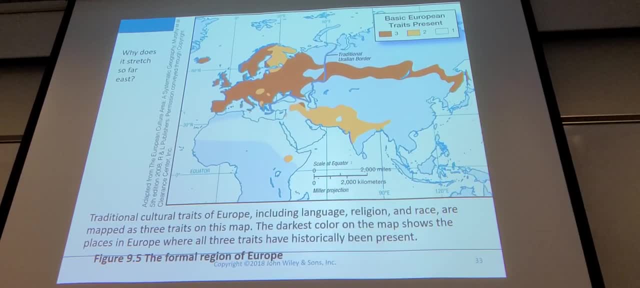 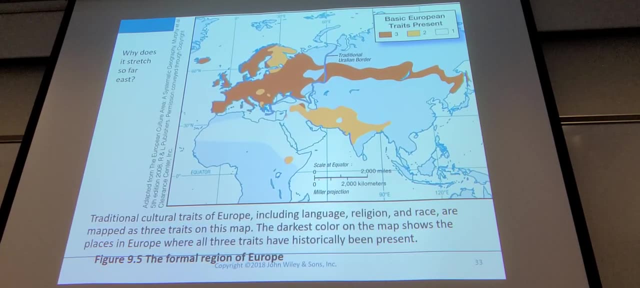 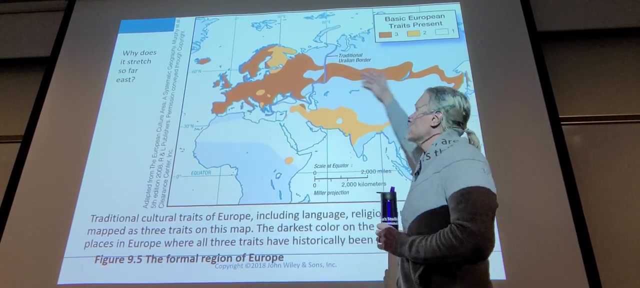 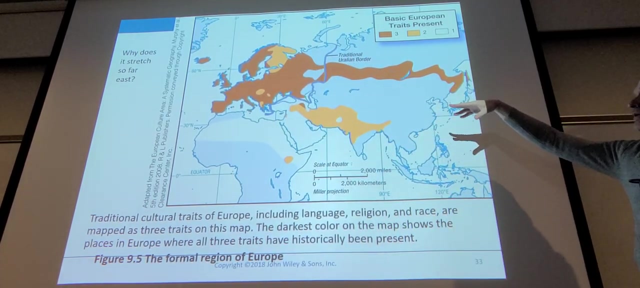 area. oh, that that is, um, that's a fair guess. but the reason these have these strong European trades isn't because of a movement this way. um, it was because of moving this way the Soviet Union, um, um, used to ship out political dissidents to this area. 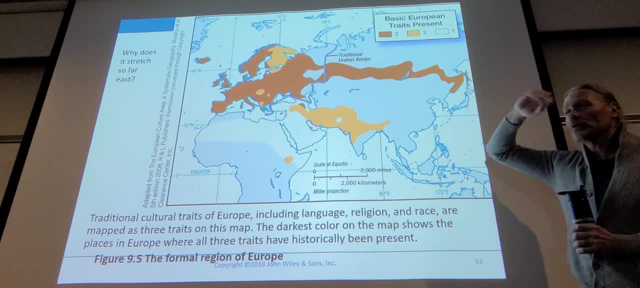 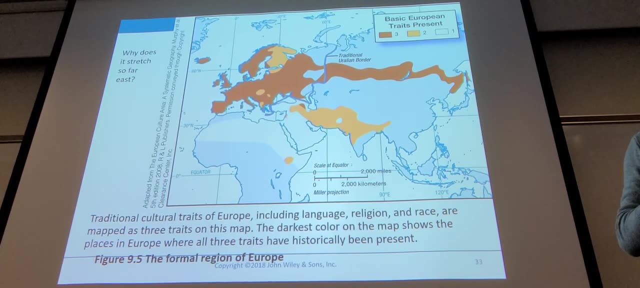 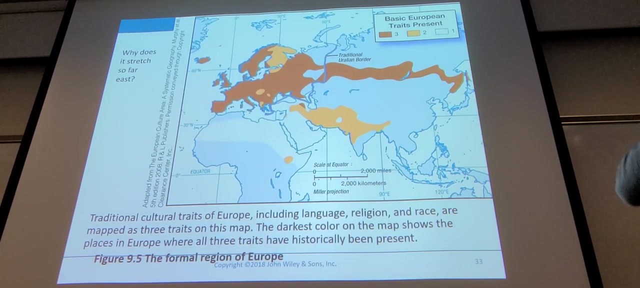 here is all along the border of China, and, if you remember, I was talking about buffer states. could anyone define a buffer state? what is the purpose of a buffer state? well, it's basically you have a powerful, maybe an empire or a country- right, and let's say you have another powerful country, that's right, but besides, 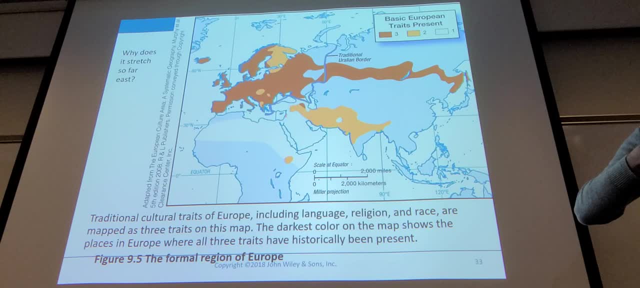 you have a powerful country that's right, but besides you have a powerful country that's right, but besides it right. and if their borders are it right and if their borders are it right and if their borders are along each other, you're really nervous that, along each other. you're really nervous that. 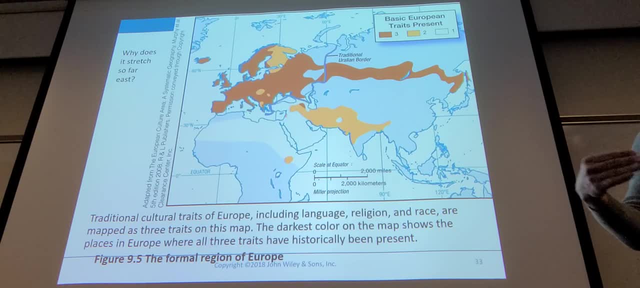 along each other. you're really nervous that the other country, if they wanted to the other country, if they wanted to the other country, if they wanted to invade, they have their military right. invade, they have their military right. invade, they have their military right there on the border. anyway, it'd be very. 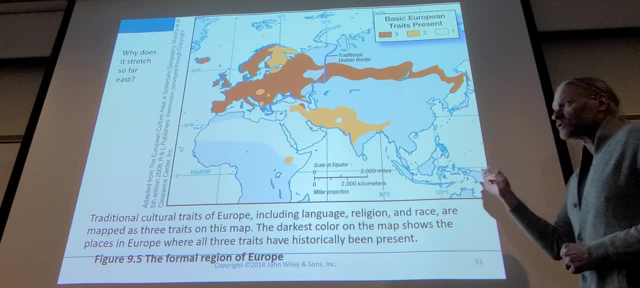 there on the border anyway. it'd be very there on the border anyway. it'd be very quick and easy for them to evade. so what quick and easy for them to evade. so what quick and easy for them to evade. so what often places will do is they'll create a. 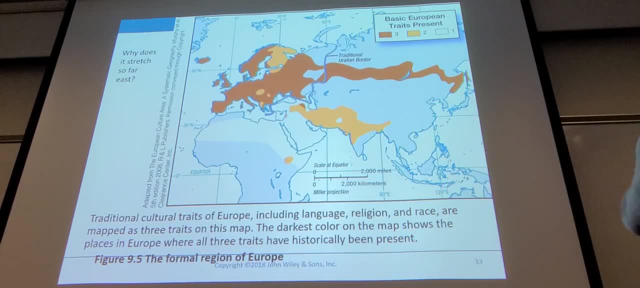 often places will do, is they'll create a often places will do, is they'll create a border state. they'll say something like border state. they'll say something like border state. they'll say something like: this is a border city for when they get. this is a border city for when they get. 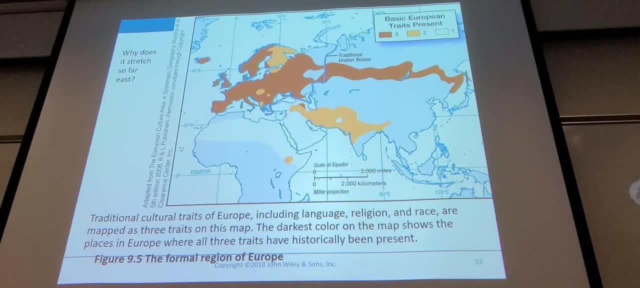 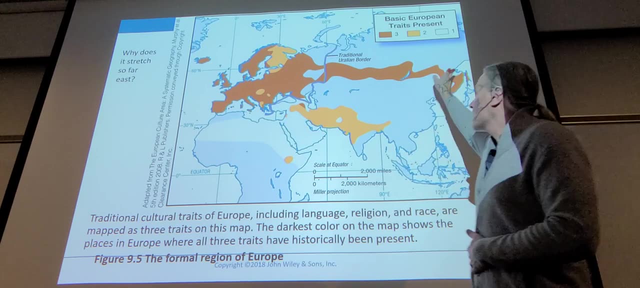 this is a border city for when they get to us um Mongolia. yeah, those are good to us um Mongolia. yeah, those are good to us um Mongolia. yeah, those are good examples of buffer states, and that's you examples of buffer states, and that's you examples of buffer states, and that's you know all along here. and so Union is. 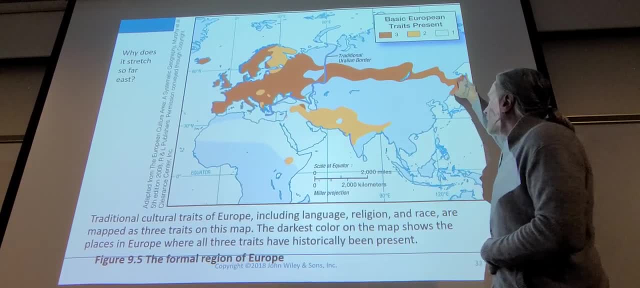 know all along here, and so Union is know all along here, and so Union is trying to basically make another. well, trying to basically make another well, trying to basically make another. well, they didn't want to have this area, not, they didn't want to have this area, not. 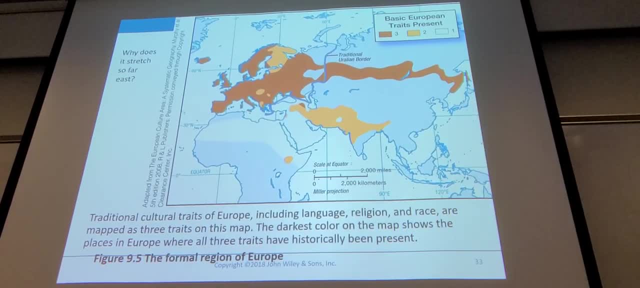 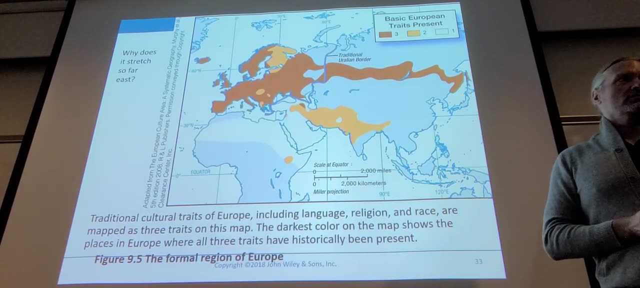 they didn't want to have this area not have people from Russia, right? this is a have people from Russia, right. this is a have people from Russia, right. this is a part of the larger, larger part of the larger, larger part of the larger, larger Russia: Russification, Russification, that's. 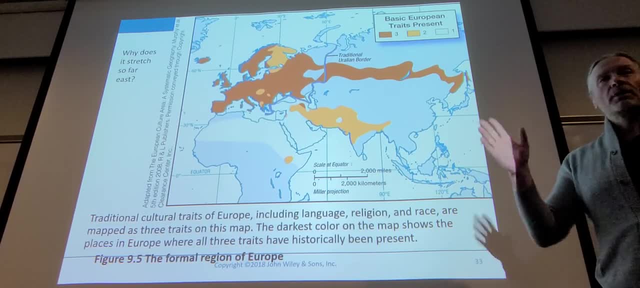 Russia, Russification, Russification. that's Russia, Russification, Russification. that's actually a term that doesn't come up, actually a term that doesn't come up, actually a term that doesn't come up into the next chapter, but I'm going to into the next chapter, but I'm going to. 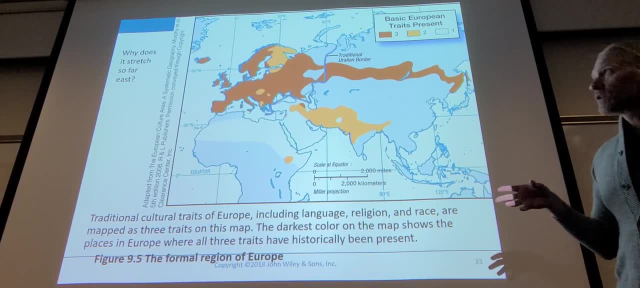 into the next chapter, but I'm going to describe it anyway because it comes up, describe it anyway because it comes up, describe it anyway because it comes up and it's and it's relevant Russification, and it's and it's relevant Russification and it's and it's relevant. Russification is a term for something that all 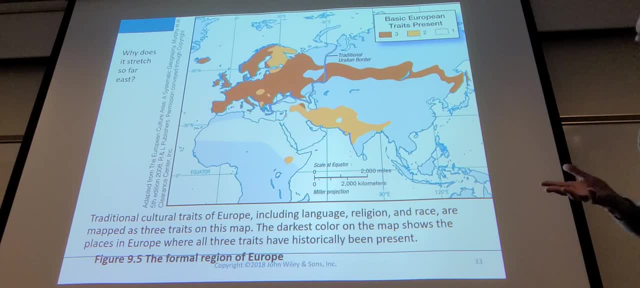 is a term for something that all is a term for something that all empires did. Russification was right. you empires did Russification was right. you empires did Russification was right. you know the Soviet Union a whole bunch of. know the Soviet Union a whole bunch of. 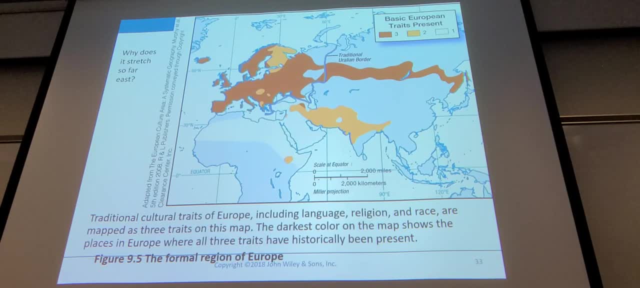 know, the Soviet Union, a whole bunch of different countries, different languages, different countries, different languages. different countries, different languages, different ethnicities- right, but Russia, different ethnicities, right, but Russia, different ethnicities, right, but Russia is in charge and in control. well, what is in charge and in control? well, what? 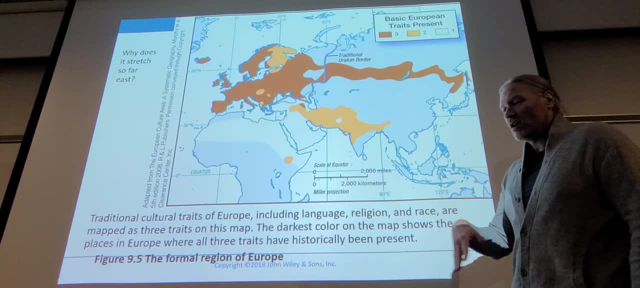 is in charge and in control. well, what they did was places that they had. that they did was places that they had. that they did was places that they had that they were in charge and control of they. they were in charge and control of they. they were in charge and control of they wanted those places to well speak. 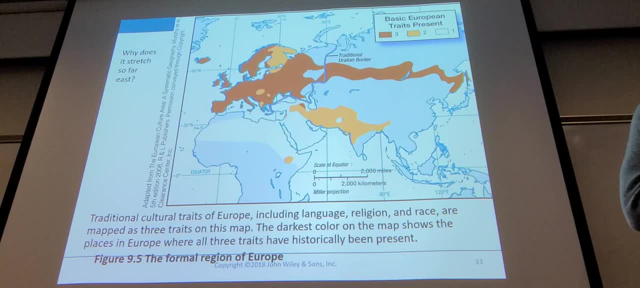 wanted those places to well speak, wanted those places to well speak Russian right and take out Russian Russian right and take out Russian Russian right and take out Russian values. so imperialism isn't just about values. so imperialism isn't just about values. so imperialism isn't just about economic and taking over an area and 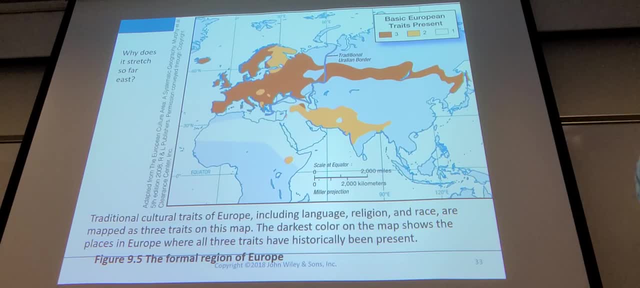 economic and taking over an area, and economic and taking over an area and taking their resources. but it's usually taking their resources, but it's usually taking their resources, but it's usually about it's a cultural thing it's about. about it's a cultural thing it's about. 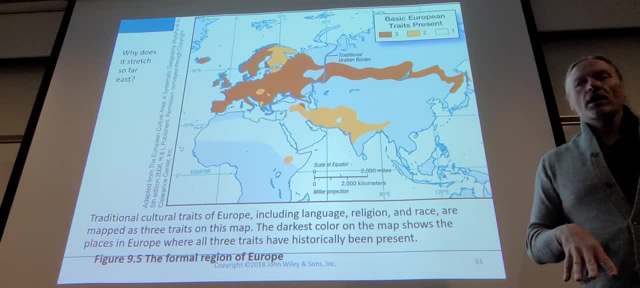 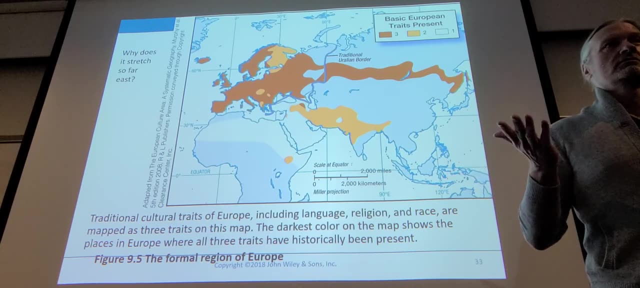 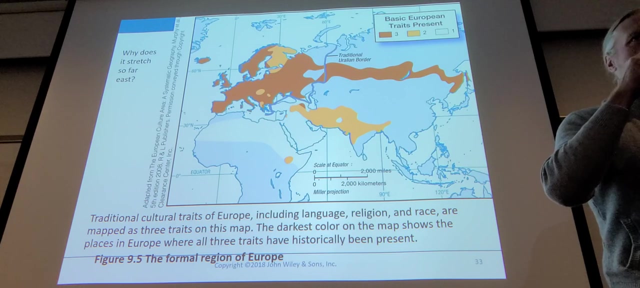 about. it's a cultural thing. it's about getting rid of those other cultures, getting rid of those other cultures, getting rid of those other cultures completely. people ever study history completely. people ever study history completely. people ever study history. heard of Prussia, Prussia. where is Prussia? 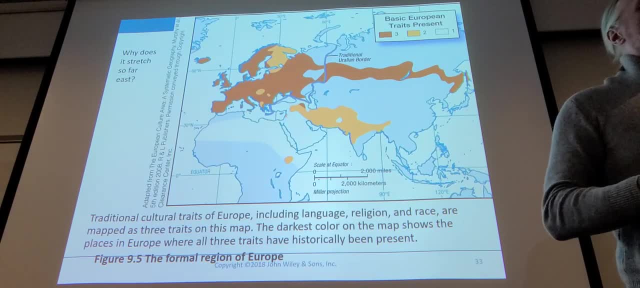 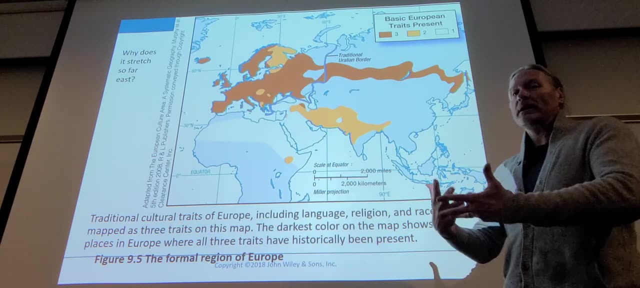 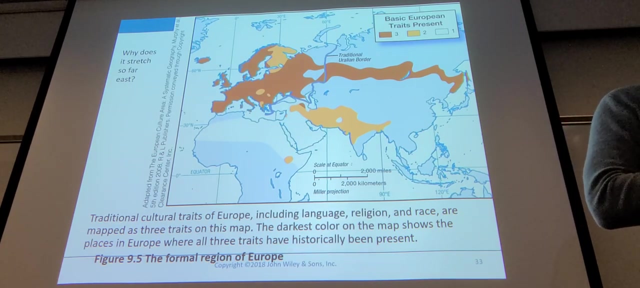 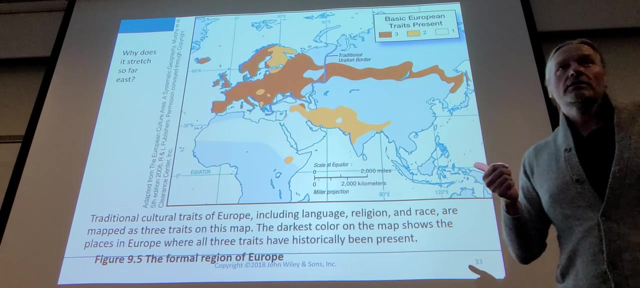 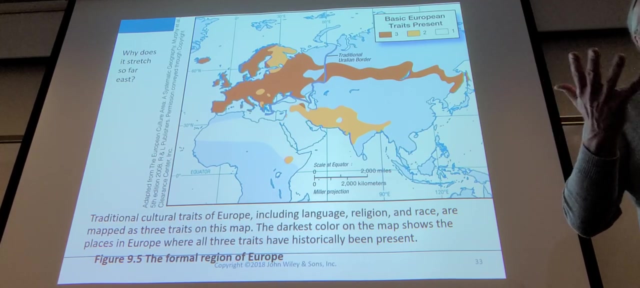 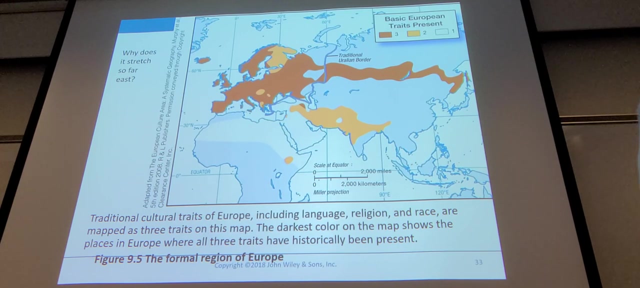 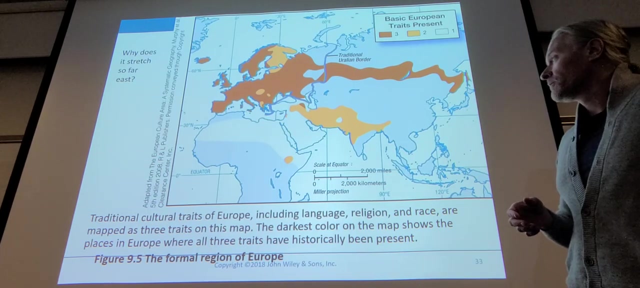 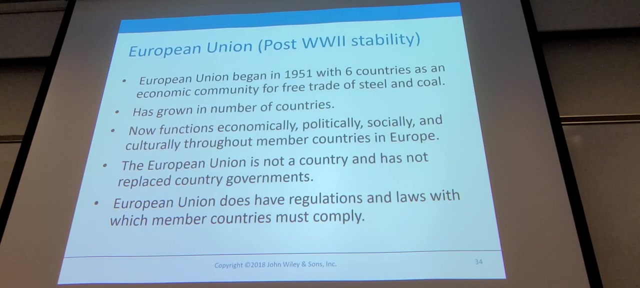 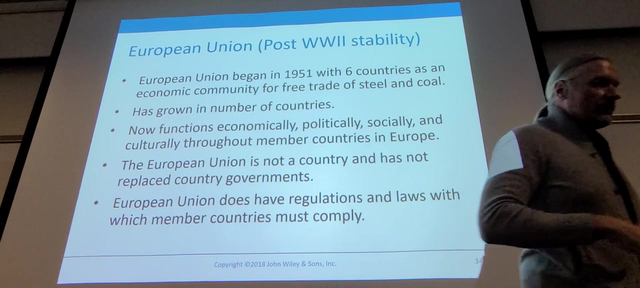 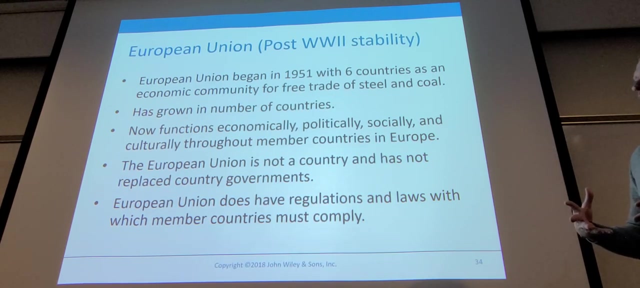 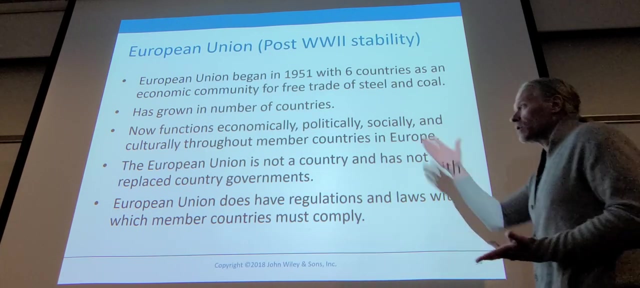 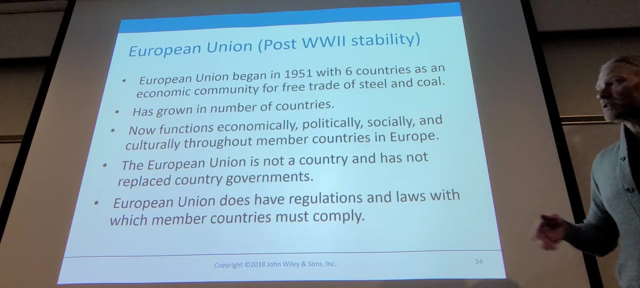 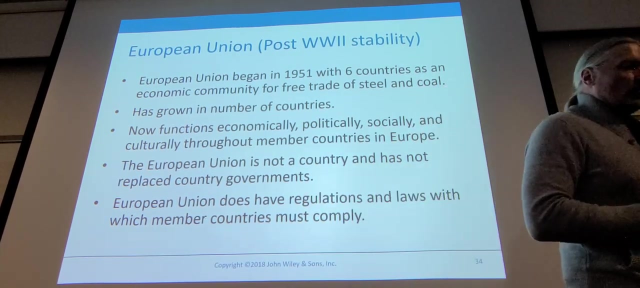 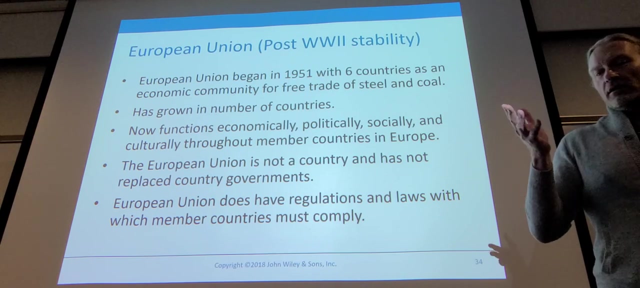 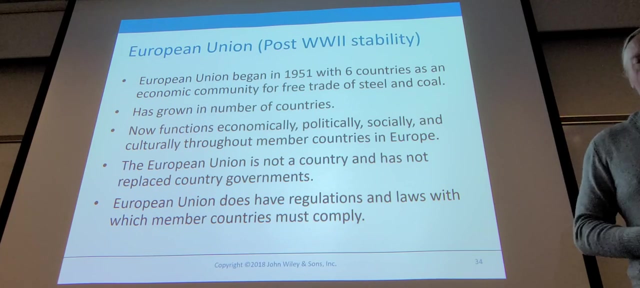 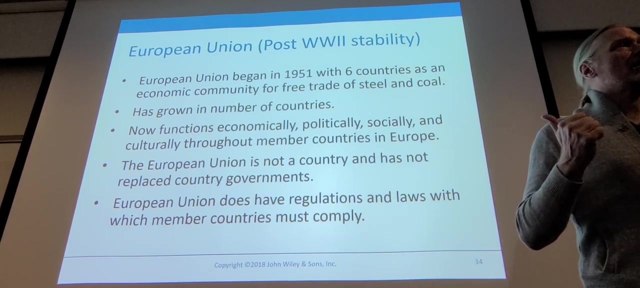 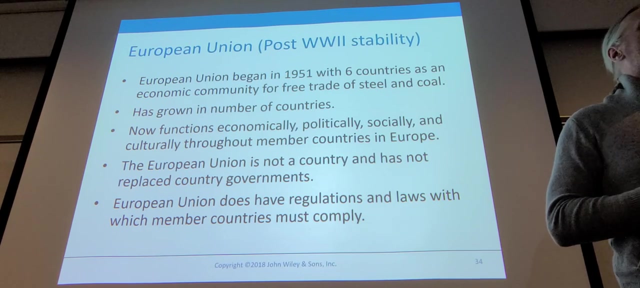 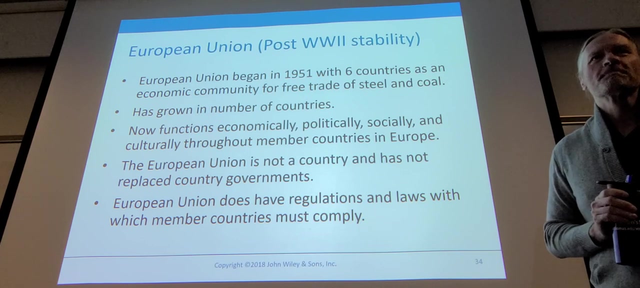 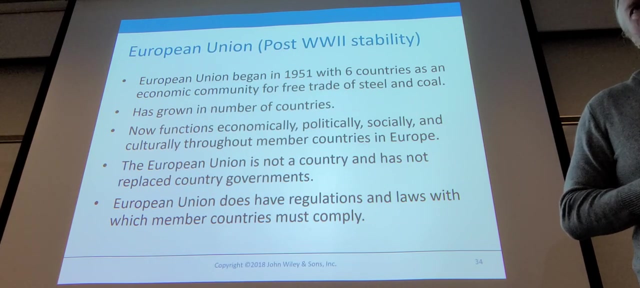 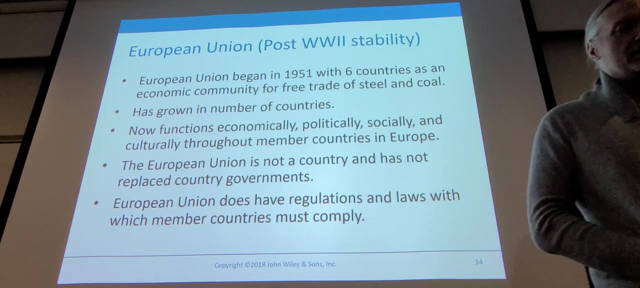 yes, yes, yes. it's one of those things where the yes. it's one of those things where the yes. it's one of those things where the different, different countries will have these old kind of battles right that are previous. countries will have these old kind of battles right that are previous. 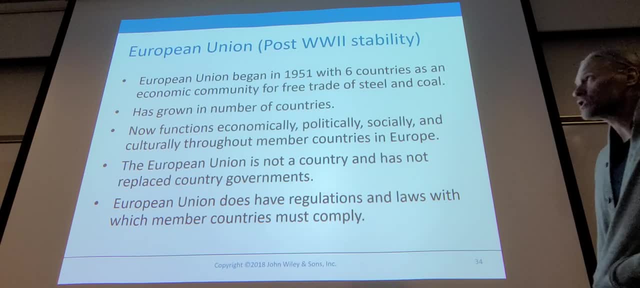 countries will have these old kind of battles right. that are previous generations, that in some ways new generations, that in some ways new generations, that in some ways new generations will try to move on from like generations will try to move on from, like generations will try to move on from like. there's plenty of people who consider 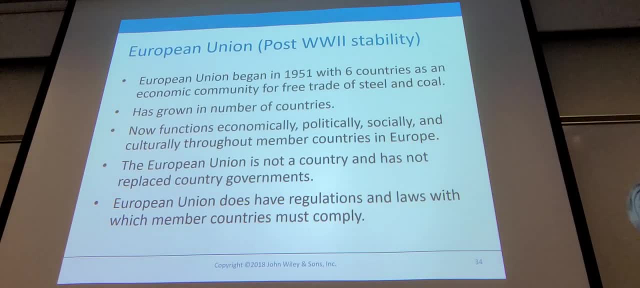 there's plenty of people who consider. there's plenty of people who consider the European Union to be the future and the European Union to be the future and the European Union to be the future and to think of themselves as a European. to think of themselves as a European. 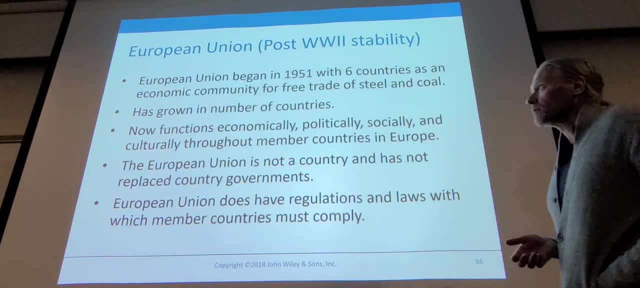 to think of themselves as a European rather than a specific German, or a rather than a specific German, or a rather than a specific German, or a different country, right. but then you have different country, right, but then you have different country, right. but then you have plenty of people who hate all that. 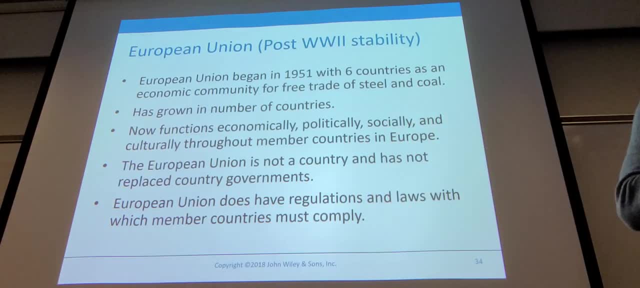 plenty of people who hate all that, plenty of people who hate all that, and they well, they think that their and they well, they think that their and they well, they think that their culture is vastly superior to others and culture is vastly superior to others and culture is vastly superior to others and they actively dislike even others. 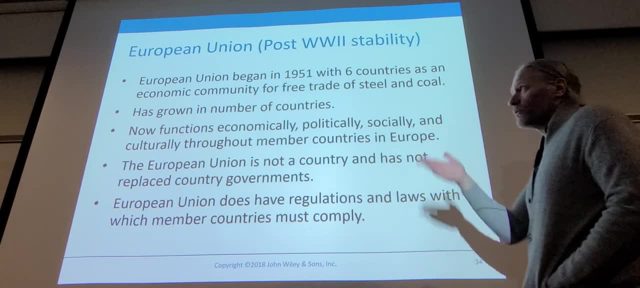 they actively dislike even others. they actively dislike even others within their own country. that if we were within their own country, that if we were within their own country, that if we were visiting. you know if you visit Germany visiting. you know if you visit Germany visiting. you know if you visit Germany, for example, like you go to one region. 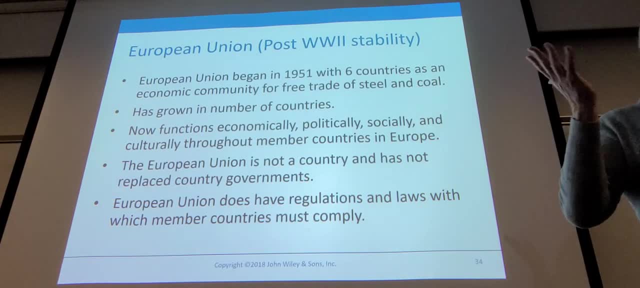 for example, like you go to one region. for example, like you go to one region and it may seem very similar to the next, and it may seem very similar to the next and it may seem very similar to the next, right like the customs are just slightly right, like the customs are just slightly. 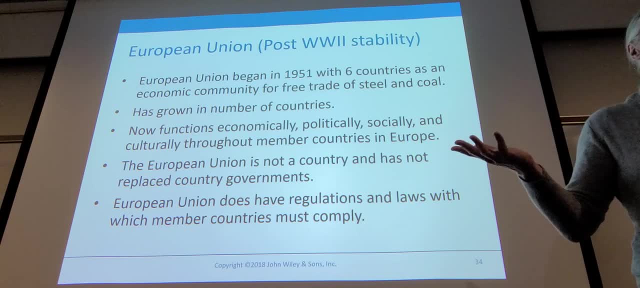 right, like the customs are just slightly different between: and you know I'm a different between- and you know I'm a different between: and you know I'm a geographer who studies cultures and I'll geographer who studies cultures and I'll geographer who studies cultures and I'll go to places. I'll be like I had no idea. 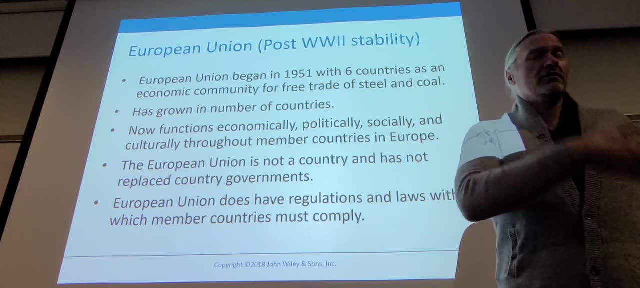 go to places, I'll be like I had no idea. go to places, I'll be like I had no idea that this is a different type of people, that this is a different type of people, that this is a different type of people over here and it's over here, you know. 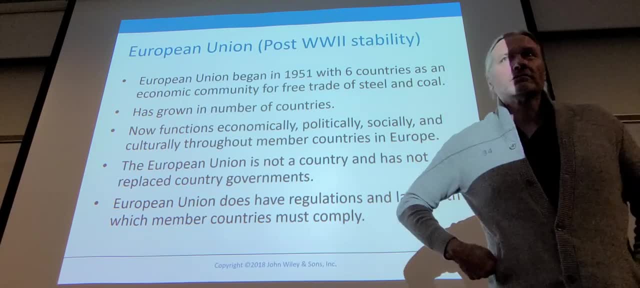 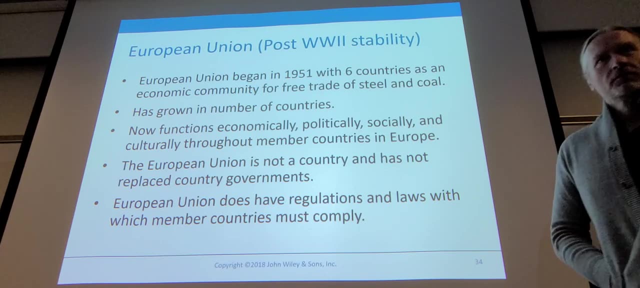 over here and it's over here. you know, over here and it's over here. you know, it all seemed similar to over here and it all seemed similar to over here, and it all seemed similar to oh yeah, oh yeah, oh yeah. and now it's kind of like: okay, yeah, we're. 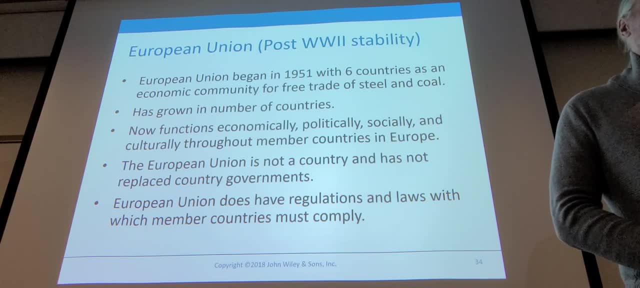 and now it's kind of like, okay, yeah, we're. and now it's kind of like, okay, yeah, we're so progressive in the wonderful this, that so progressive in the wonderful this, that, so progressive in the wonderful this, that will be good. well, it depends on which ones, though. well, it depends on which ones, though. well, it depends on which ones, though. right, there's there again. like I said, right, there's there again. like I said, right, there's there again. like I said, there are plenty of people who have. there are plenty of people who have. 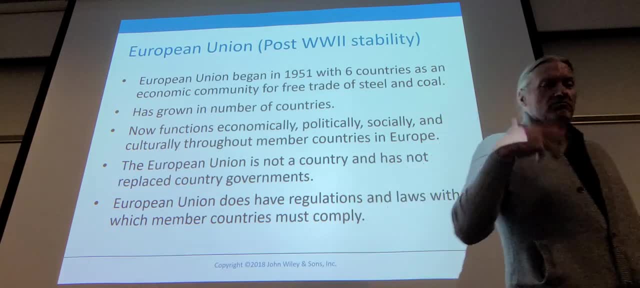 there are plenty of people who have decided there are a new generation. they decided there are a new generation. they decided there are a new generation. they want to move on, want to move on, want to move on. they're, they're, they're, they're, they're, they're, they're like other Europeans. and then there's 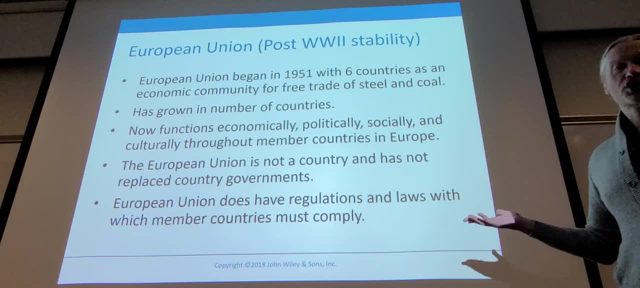 like other Europeans, and then there's plenty of people who don't right. the ratio of those types of people in the countries it might be like 50-50, and so when you're running around and you meet people, you'll meet lots of different types. oh, let me just finish up on this. 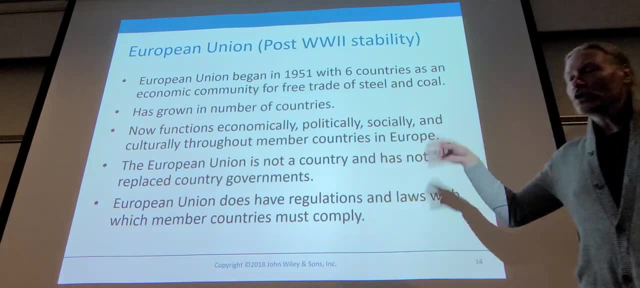 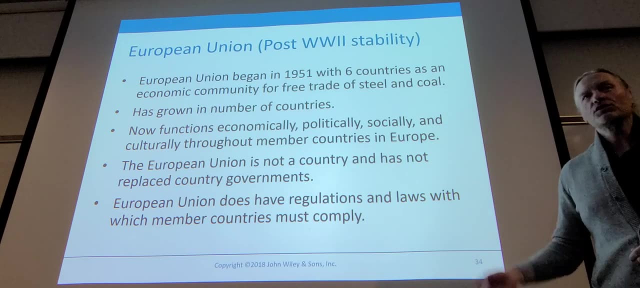 subtopic topic. so after the European came together, right, it was mostly an economic union at first, but this made it so that, like, let's say, you just wanted to have start up a light bulb company, right and well, you just want to have a standard for like the socket that you're gonna put a light bulb button and be. 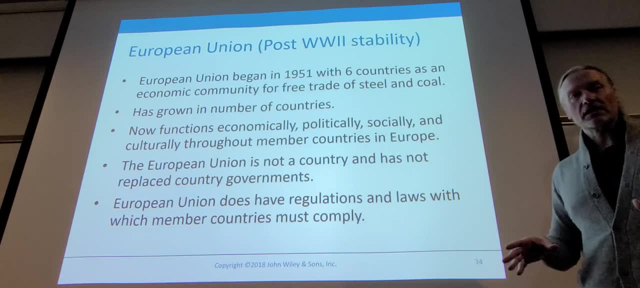 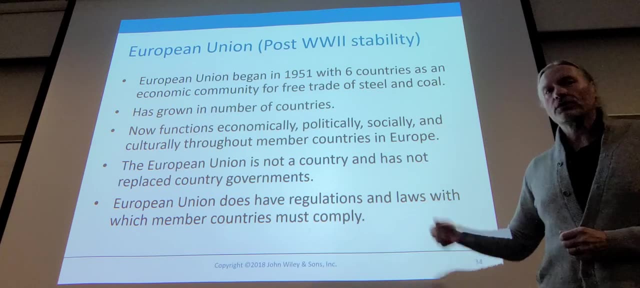 able to sell it to different countries. well, they started standardizing these things so you could. you would have the whole European market instead of just a small country. for travelers it's much easier to just kind of go around and around to different countries than I used to be. right, don't have to check. 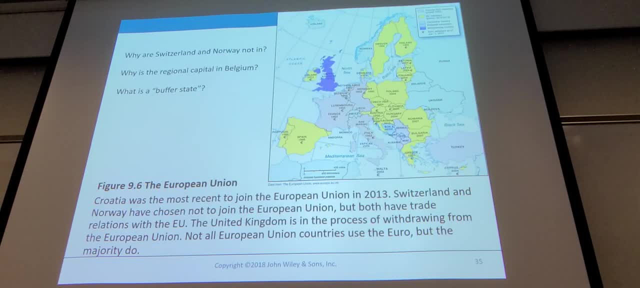 your passports and go through a big thing. so map of the European Union. see a lot going on here. these are different years that the different countries became parts of the European Union. you'll notice some countries that are not part Norway. right now Norway is definitely like in Europe, so you want to know why Norway would not want to be in the 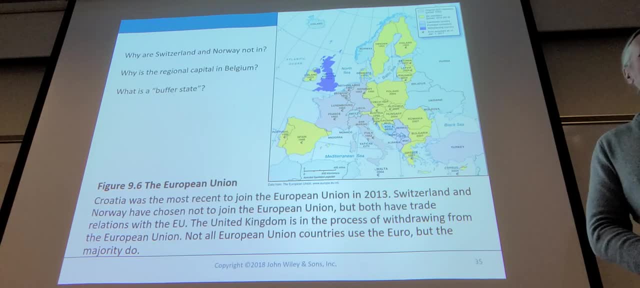 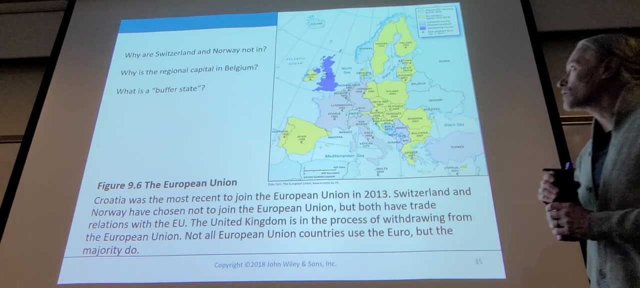 European Union. first, they are kind of the border, especially right now, between Europe and Russia, and that's all true. but Norway doesn't really have too much part of that stuff. it's more money, oh sure. yeah, a whole bunch of oil has been found in the nrc here right now, when you're part of the 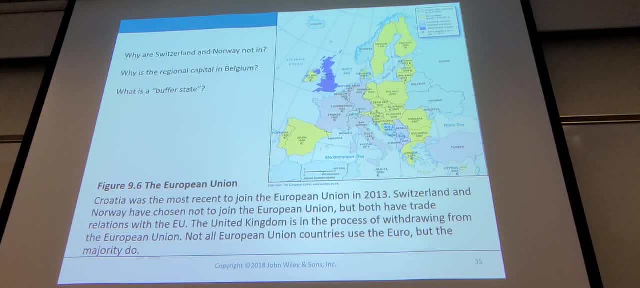 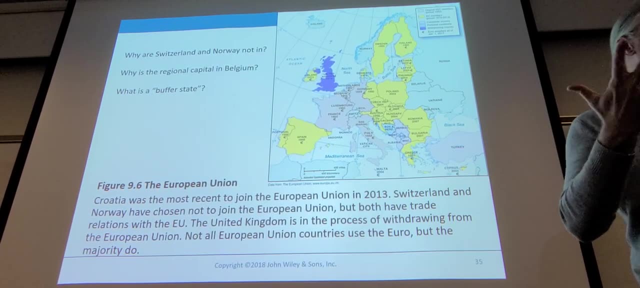 european union. it's just like you know, if you're a state within the united states, you're paying taxes, you're paying federal taxes, right? um, there's lots of states who have a bit of an attitude of like, well, all that money should stay in my state because it's going to all these other states that 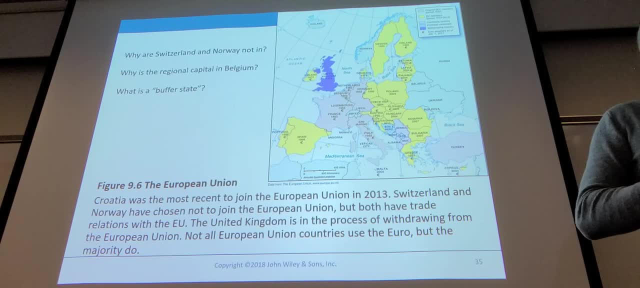 are- i don't know what's going on in those states- right, and if you have countries, they have even more of that kind of a feeling. so norway spends uh well, if you remember different countries that were having trouble with their birth rates. so they want to put in a lot of benefits to people. to have kids. that stuff costs money. norway actually has a real great uh social safety net, uh for all kinds of different things- retirement, having kids, you name it uh, and part of the reason is because they have all this oil money. uh, if they became part of the european union. 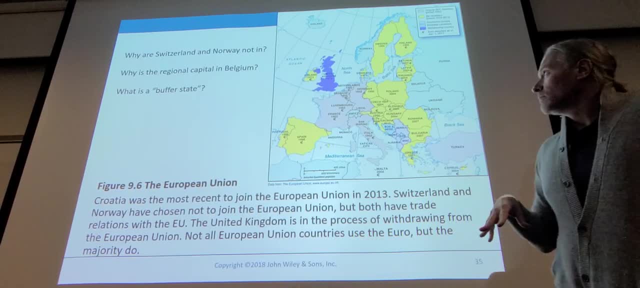 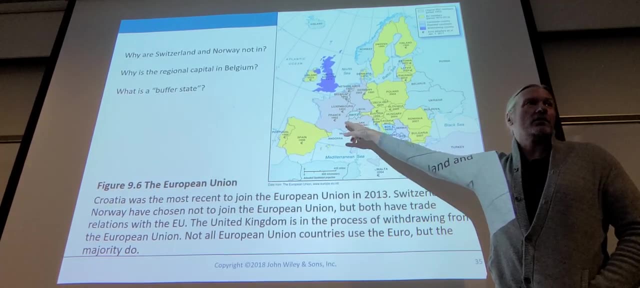 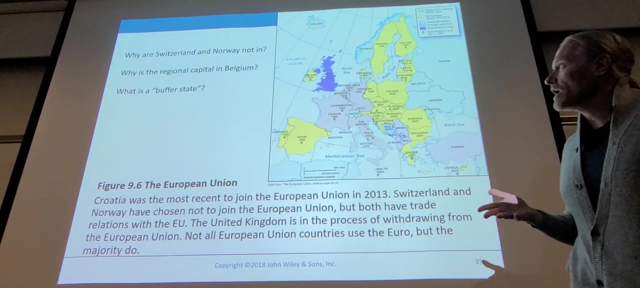 they'd have to share that around more, right? um, switzerland also not part of the european union? uh, why would that be? why would switzerland? there's a few different reasons. what's that? they have historically said that they're neutral in different things and wars and whatnot. 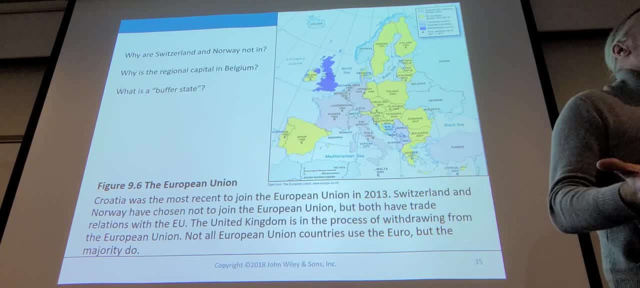 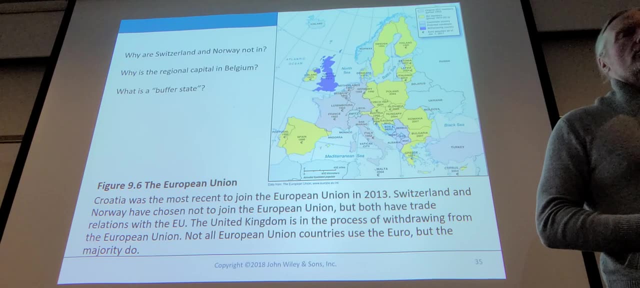 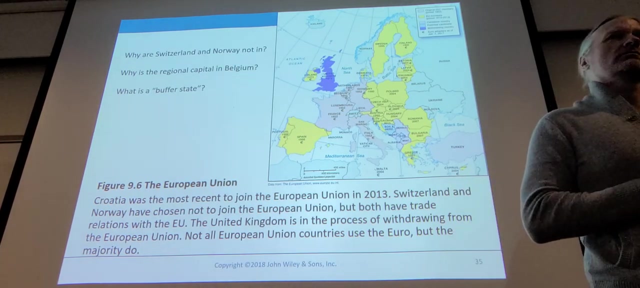 but there's a bit of a reason why they stress that neutrality. is there a way for them to make money on their neutrality? united nations- we're talking before before that they're a safe haven for people to store their money. they'll take in money from anyone. 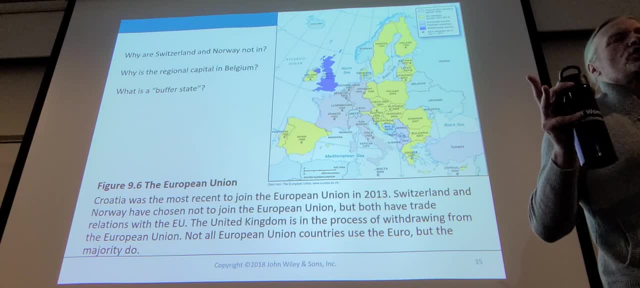 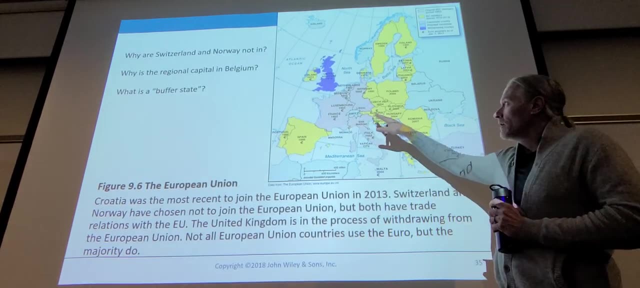 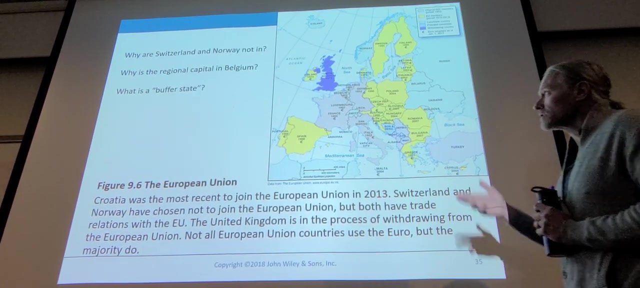 swiss bank accounts. right, you probably heard of that. turn use sometimes like: oh, secret swiss bank accounts. if they became part of the european union, their businesses would then be under european regulations. those european regulations would be like: oh, let's, let's take a look at these. 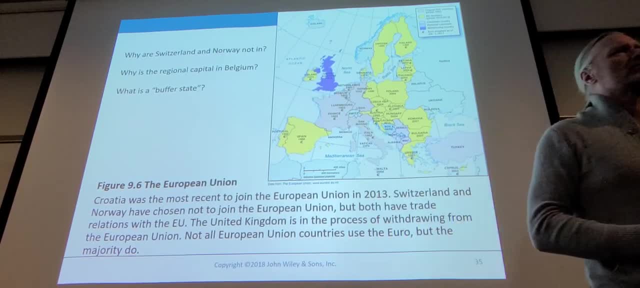 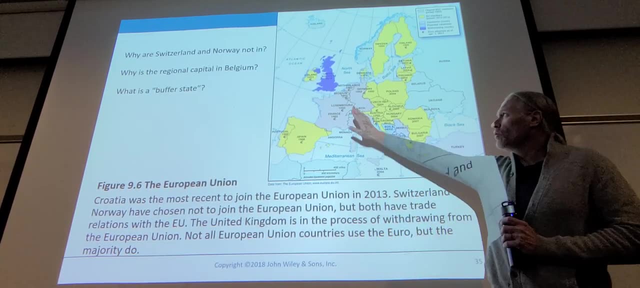 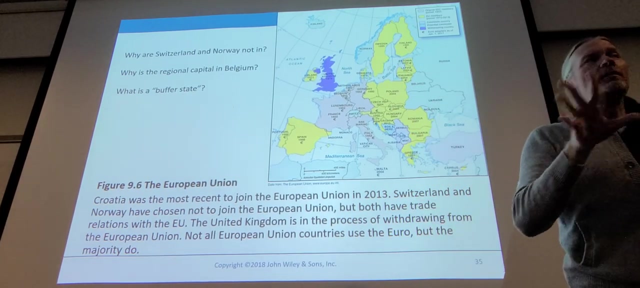 bank accounts and just see what's happening. where's this money coming from? it's like, oh, drug lords in different areas of the world, um right, old nazi money, a huge range of money that are in secret bank accounts that switzerland doesn't really want people playing their eyes into right and checking out they. they want all that stuff to be just kind. 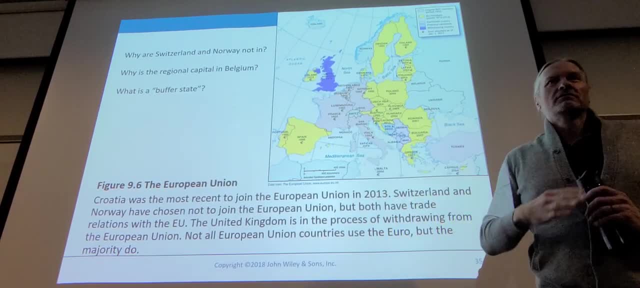 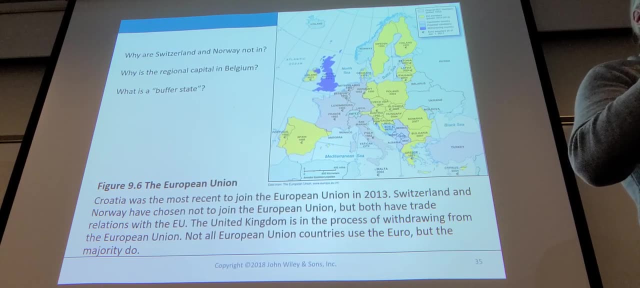 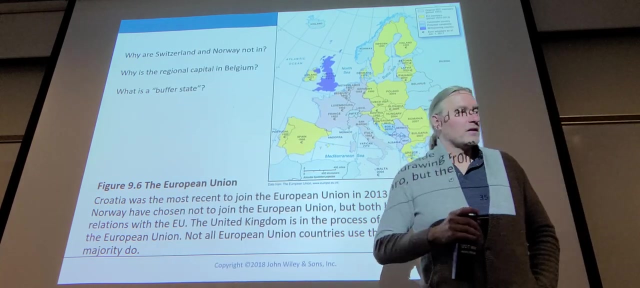 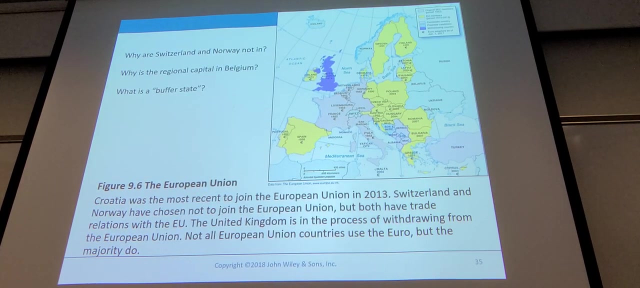 of kept kept their little secret. yeah, like your food has come back. if you read about the panama papers, all right, panama papers won't go into it, but uh, yeah, there's a lot of illegal money that's being stored in places laundered, as they say, um switzerland. see if there's any other country of. 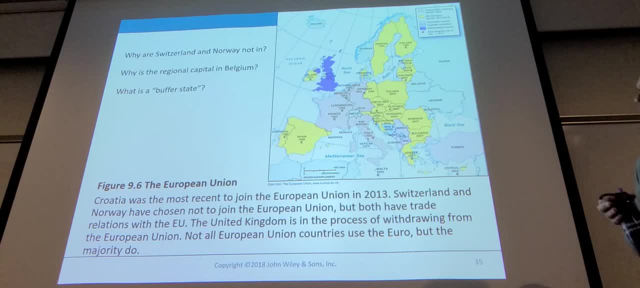 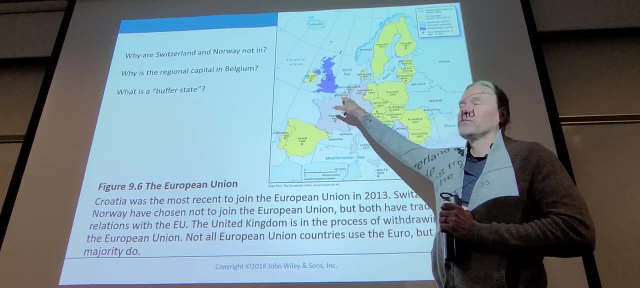 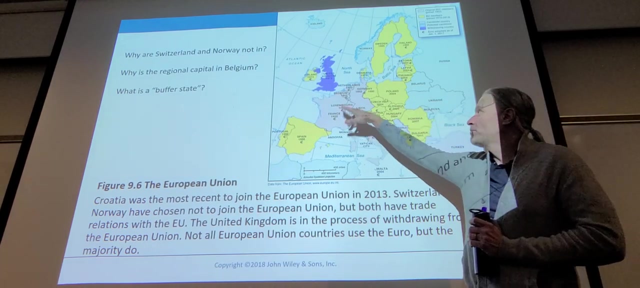 notes: um, no, that's pretty good. oh, we'll talk about buffer. oh, actually, i will mention belgium. is a classic case of a buffer state. um, belgium should just technically be part of france, um, but it's a buffer state. it was created just so if, if either country invaded this way, they would have a buffer state. 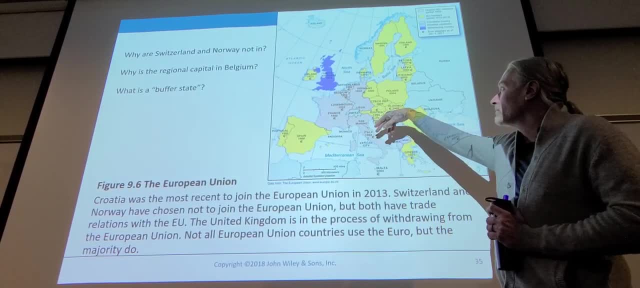 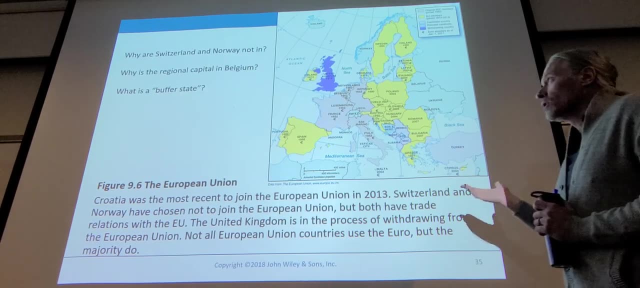 in this way, they would have countries in their way. right now, belgium is actually. this has been a bit of a benefit to belgium in modern day, because when they were looking for where would the capital of the european union be? uh, you know, there are plenty of countries that wanted it to be within their 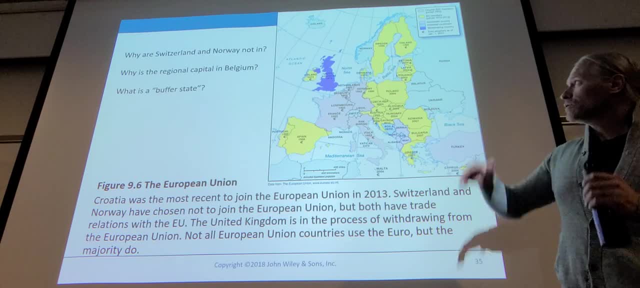 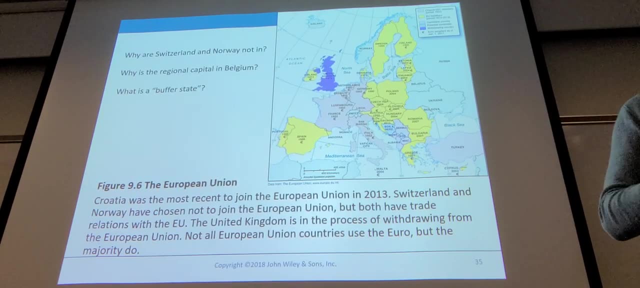 country, but if you have the entire european union. let's say you decided the capital was going to be france. well then, everything has a very french kind of. it's almost like france was the capital of europe in a way. right. so if they picked france, which was the capital of europe, they would have to 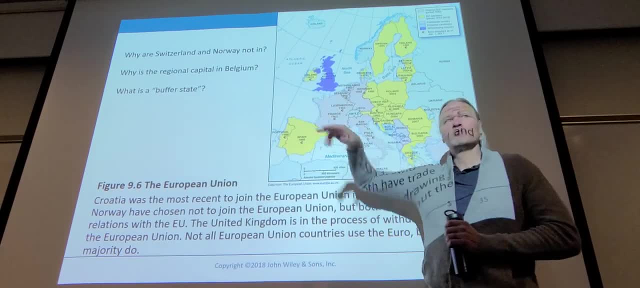 rich content and less more orange food over there as our country. that's like a few countries in another way, right. so if they pick france, they would have to give food for something different. so if they picked Belgium, which is a smaller country, had a lot less damage after the Second World War. 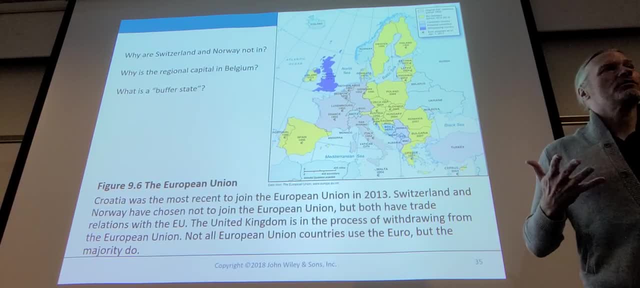 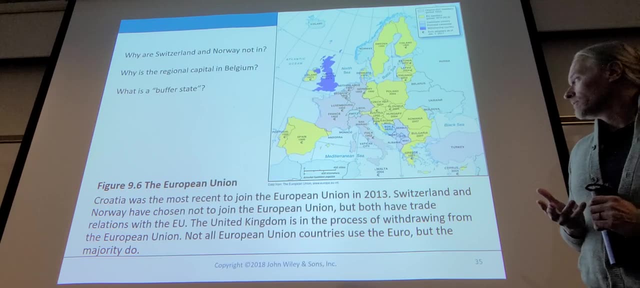 Their economy was kind of more together. Lots of things going for Belgium, and that's why Brussels is where the capital of the European Union is. Didn't Donald Trump say that it was hell? That it was what He said. it was like a hell of a place. Oh, Belgium, Wow, Their waffles are delicious. So Brexit Countries can vote to leave the European Union Like they're not forced to be in it, And so when political winds sway, or if you have a vote where not that many people show up for the vote. 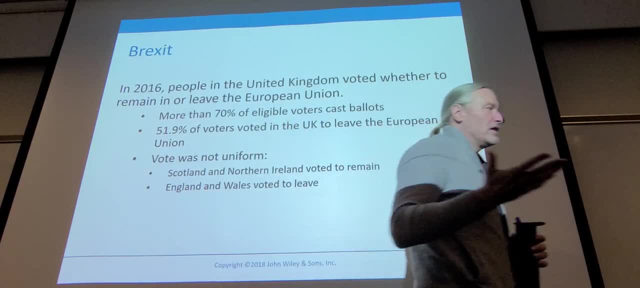 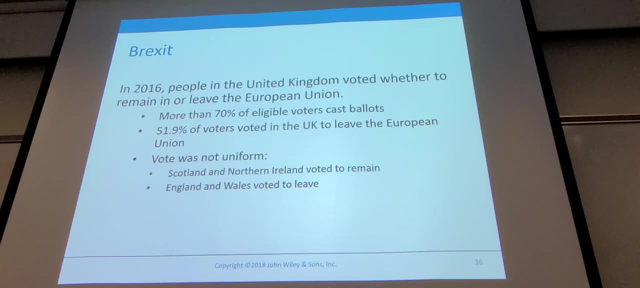 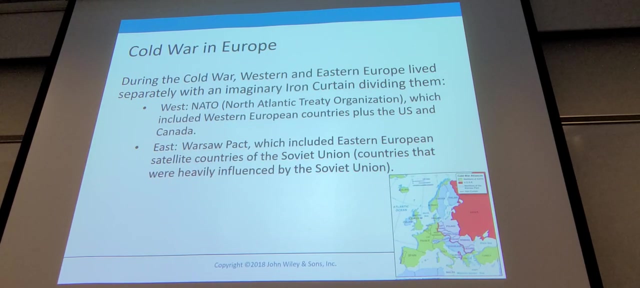 a vote is very close, but it could be something that really completely changes the economy of a place. Brexit is the term used for When the UK voted to leave Cold War in Europe, So after the video I showed you talked a lot about this right. 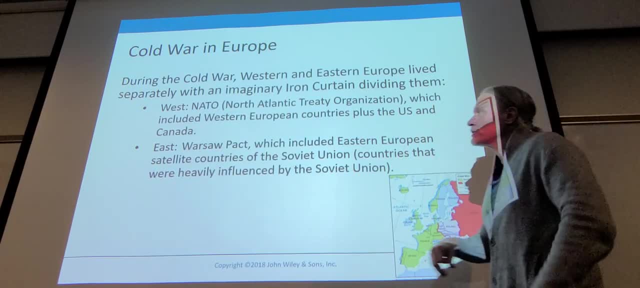 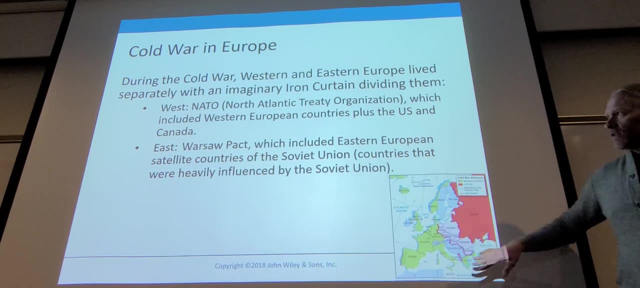 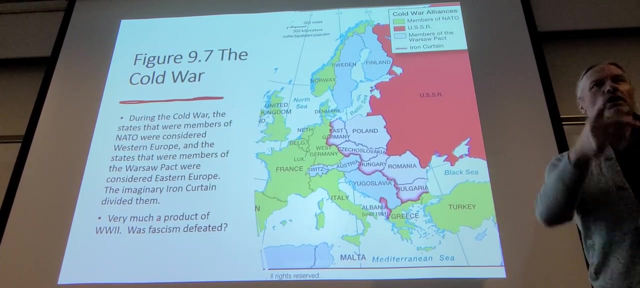 The Warsaw Pact versus NATO. The video I showed you talked a lot about NATO. I did not talk that much about the Warsaw Pact, But the Warsaw Pact was all of these different countries that were under Russian control, Yeah, So what's the difference between a Cold War and a Hot War? 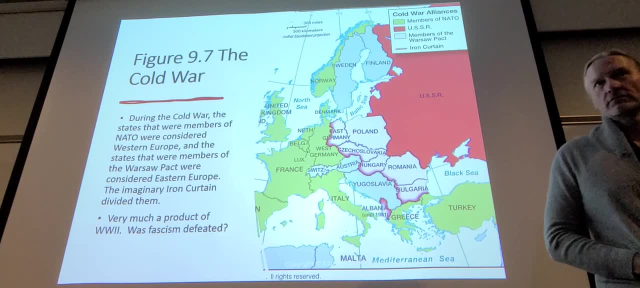 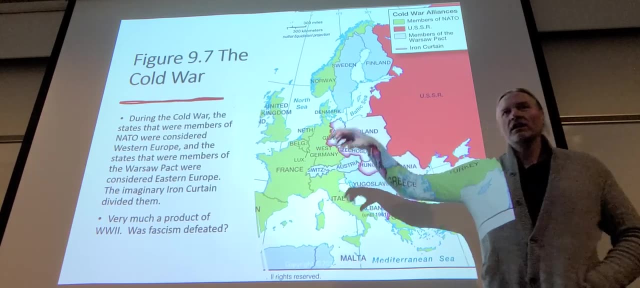 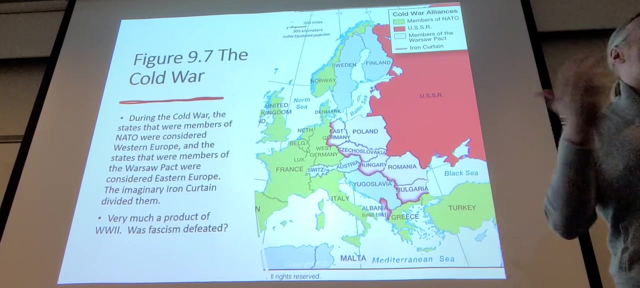 Well, that's a good question. Cold War that meant that, well, there wasn't specific military live action going on, But they had plenty of proxy wars blowing up the rest of the world. If you watch any like James Bond movies, you'll see a lot of stuff about that. 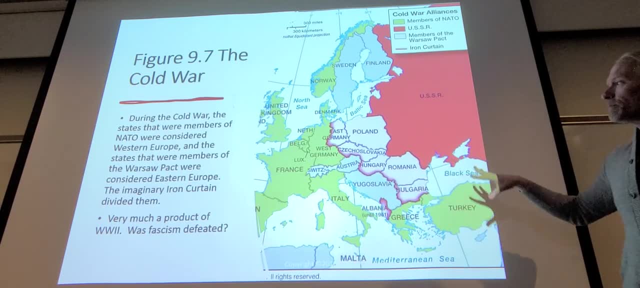 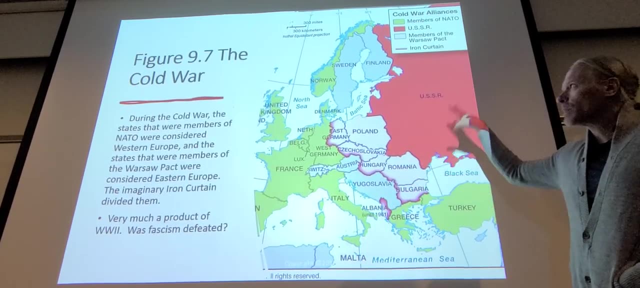 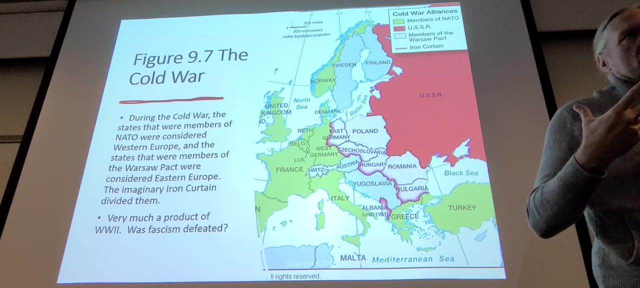 Well, and the thing was the, the, the Soviet Union tried to paint this as um as as, these being different countries that were independent but were all part of a big happy union. uh, but these countries were not part of that by choice. 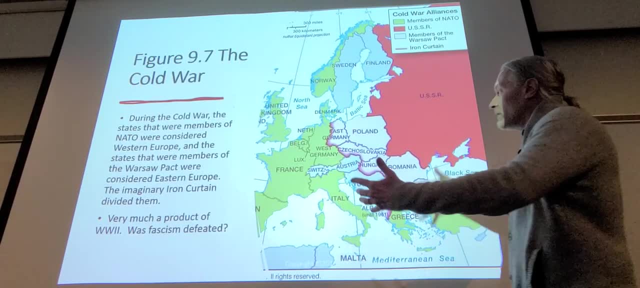 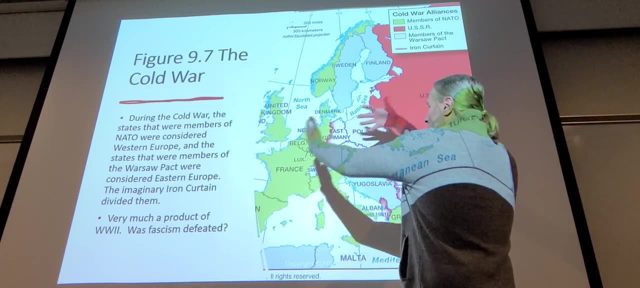 Um, at the end of the Second World War, there was a bit of a a mad dash between the different sides that were that were the winners, right? Um, and this is basically where they came together. Um, and this is basically where they came together. 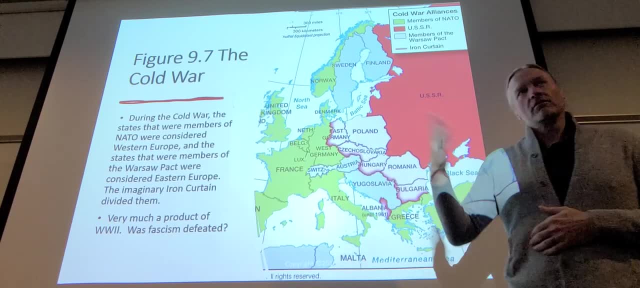 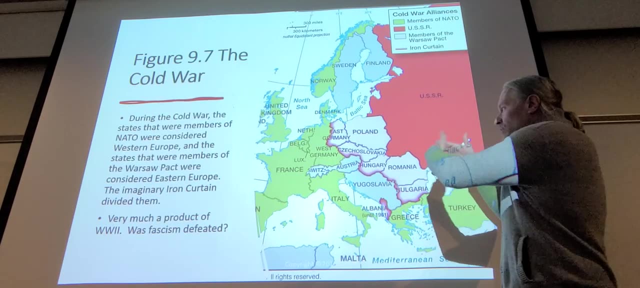 Some of these were agreed upon beforehand. There were areas of Germany that the East and West agreed that well, this is where our troops are going to meet up and this is where the new borders are going to be. Um, but a lot of it was a bit of a happenstance and kind of what happened in different areas. 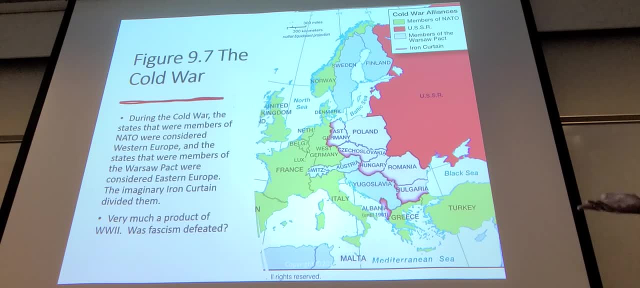 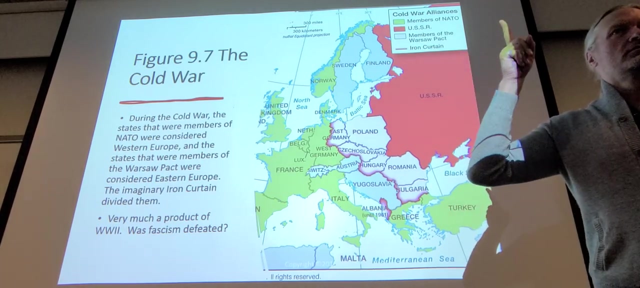 Um, Second World War is a real interesting thing, right, Because it was this fight to defeat fascism, right? Um? do you want to remember what the, what the fascist countries were? Europe In Europe, And then Italy and Japan. 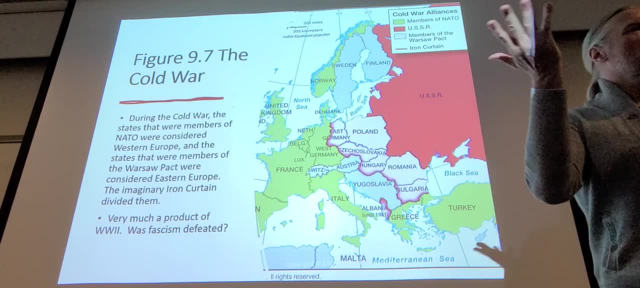 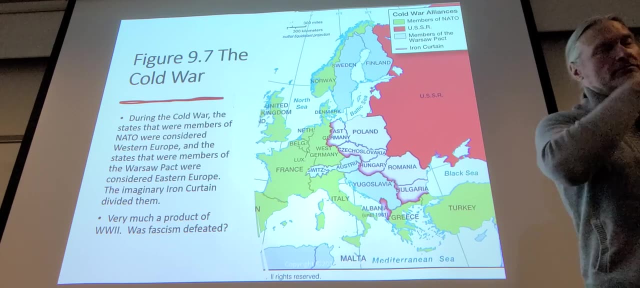 And Germany, Germany, Uh, any other countries were fascist. Yeah, Wasn't Bulgaria's leader fascist for a while? Yeah, yeah, And who else Wasn't there? um, oh God wasn't. wasn't Romania's leader fascist for a while? 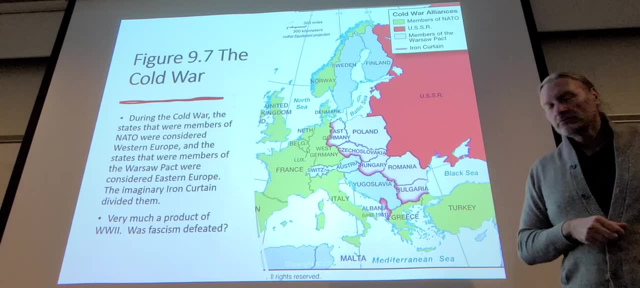 No, Or whoever Who else, be honest. But that's the thing Like sometimes it just kind of you know, like with regards to history and world politics and stuff, it's like some countries are just like the biggest. 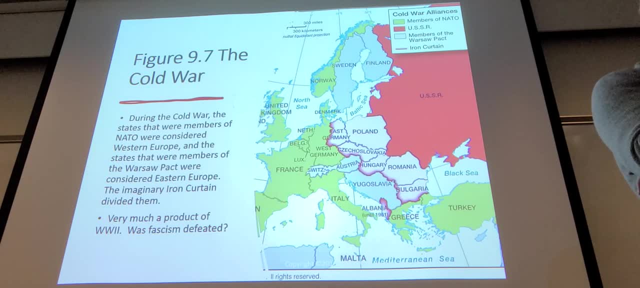 Um, you know there are biggest fighters. you know what i mean by like. you know like, for example, or mania, like, really, who gives a damn if transylvania is fascist or social? you know, um, people who live there, i mean sure, but like what? like 133 000 people who not not particularly, but like, can you understand? 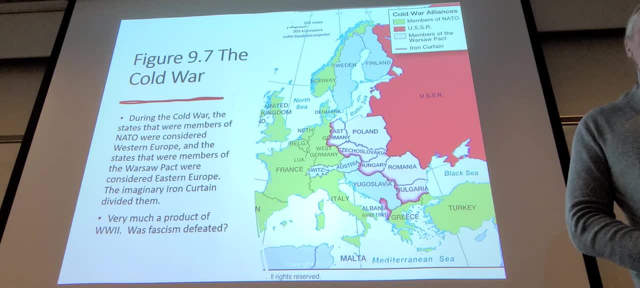 what i'm saying in the grand scheme of things, it's just like you know, it's like it's kind of like australia, you know, um, it's. it's annoying when people go out of their way to be something that they don't have to be. that makes up, for example, look at the. 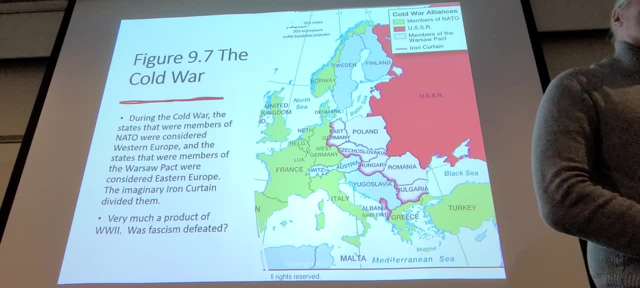 alliance with the united states and um, the alliance that just happened the other day: the united states, the uk and australia. right and now, australia is in a trade war with china, even though, if china decides to make a decisive step with regards to anything, with regards to taiwan, 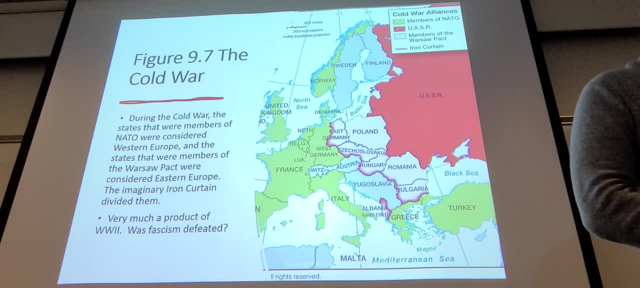 with regards to anything, then the closest person in proximity is australia. so it's kind of like sometimes it's just ties. why? because because you have colonial ties to the uk, because you have ties to the united states. but then again you think about it and it's like: okay, the uk. 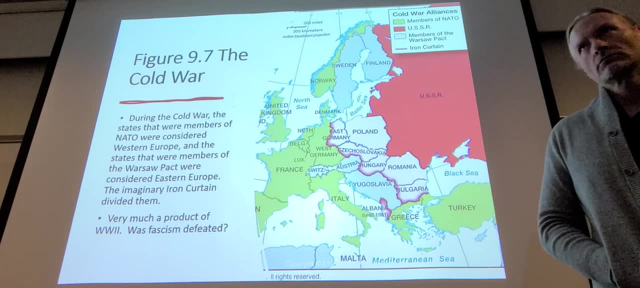 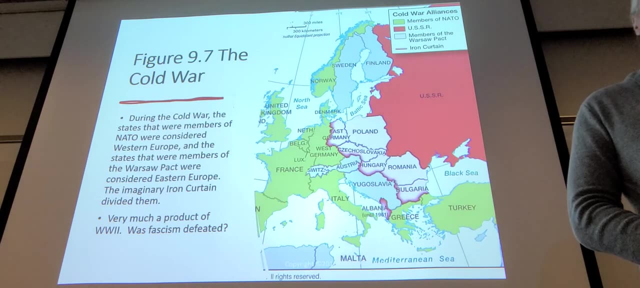 used to send everyone who is a criminal to australia. so really like, do you have ties to it or did they just treat you as criminals and expel you out of the, expelling you to somewhere where they thought it was unhappy, you know, and you guys survived. so it's really weird not to get too much. 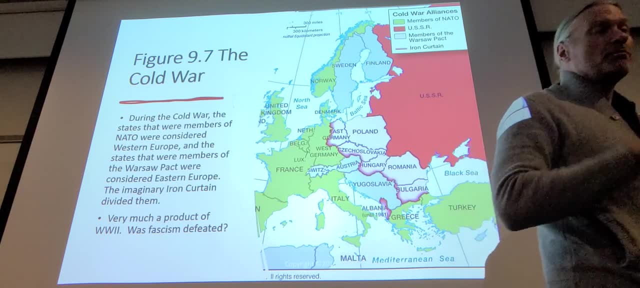 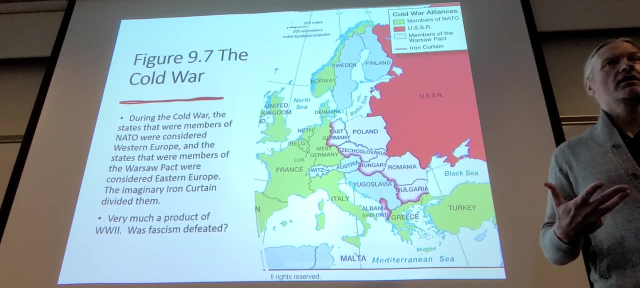 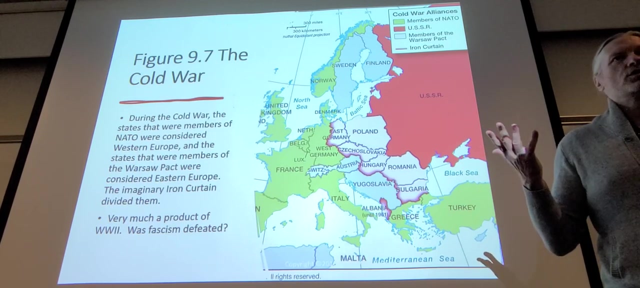 on a tangent on australia, because we'll cover australia in a couple of chapters, but i will really quickly say that it's interesting because there's a lot of people in modern day australia who feel that way. they're like: my heritage is from, you know, uh, england. but what does that have to do? 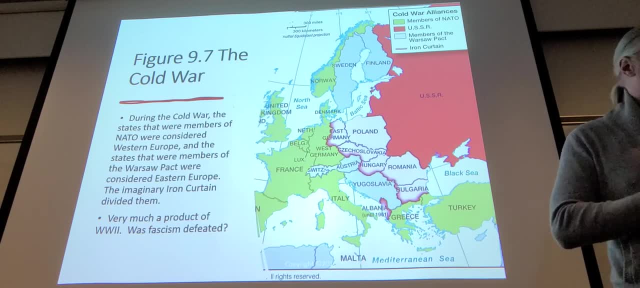 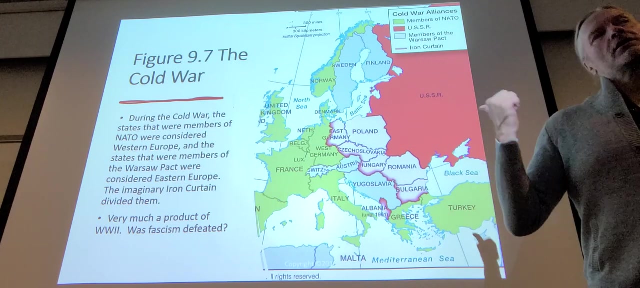 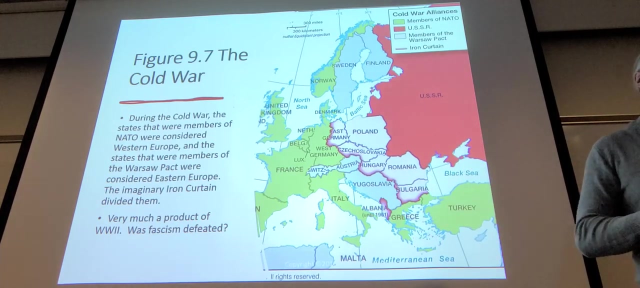 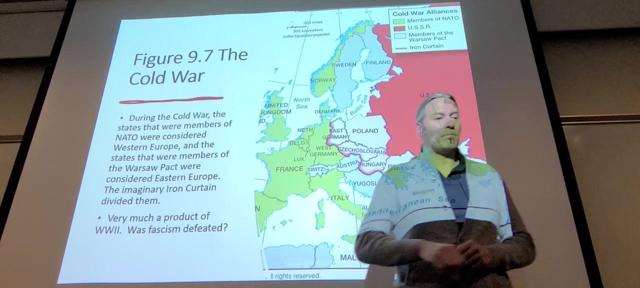 with the price of bread, exactly. well, let me backtrack to europe real quick, um, and give an example of of you know when we're talking about what other countries were fascist and what weren't, and what effect does that have on the world? if you recall, after the second world war? well, most of europe. 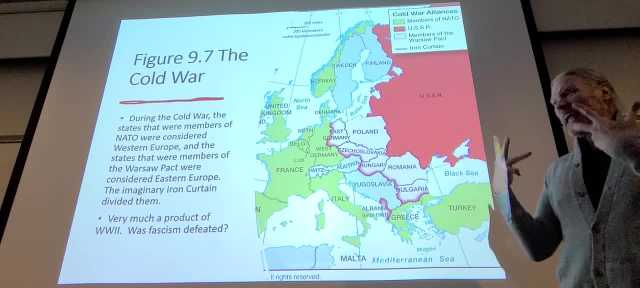 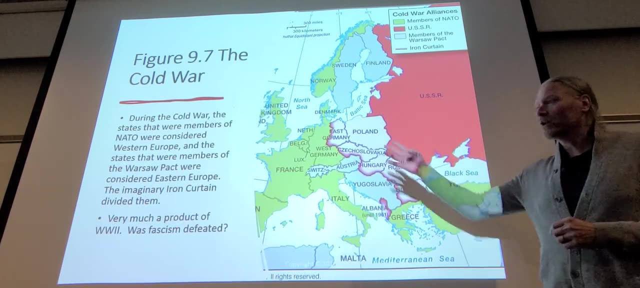 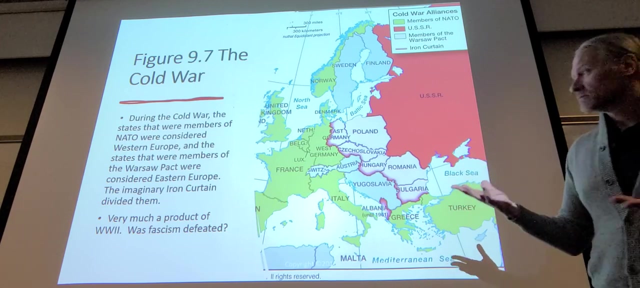 blown up. right, and that is when the age of empire faded for europe. right, that is when the post colonial time started. um was when countries switched over to being democracies. right now there are countries- oh, actually, it's not on the map here- spain and portugal. anyone know what the deal with? 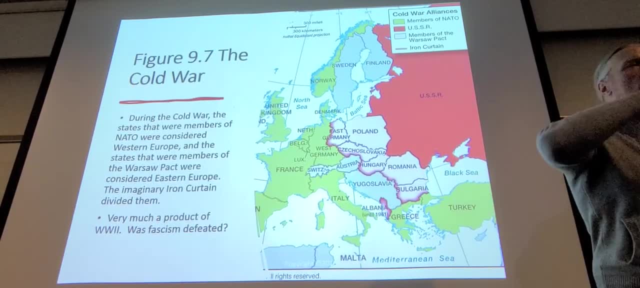 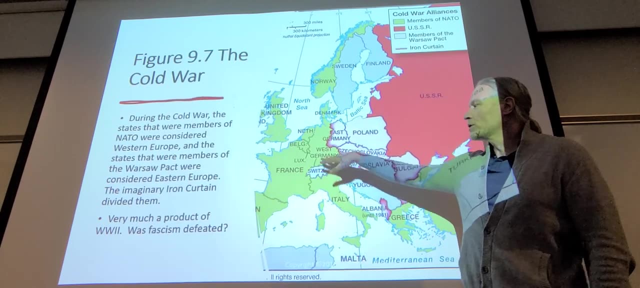 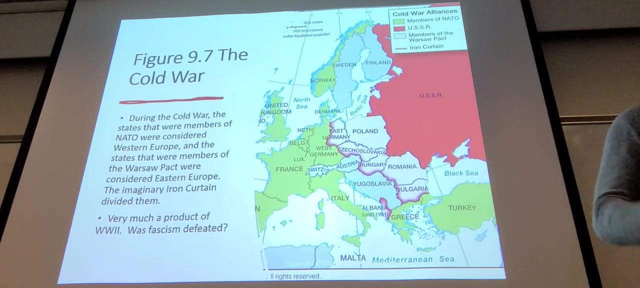 spain and portugal was during the second world war. what's that? yeah, so like we had mussolini in italy and we had hitler in germany, we had franco in spain um salazar in portugal. um, they were fascists, they helped the germans, they did all kinds of. 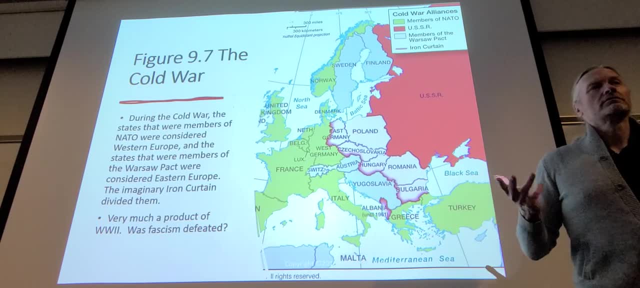 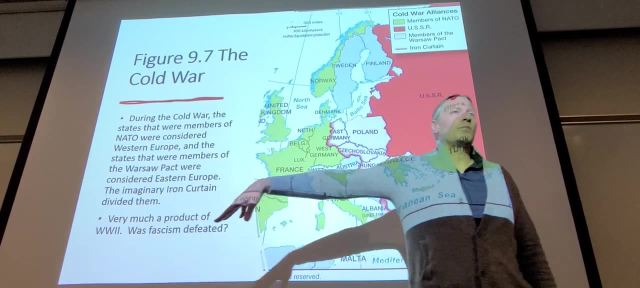 crazy stuff. now, at the end of the second world war, when we defeated fascism in europe, nobody talks about spain and portugal, because we just let them sit there. we didn't go after them, we didn't get rid of their dictators. now, what did that mean? 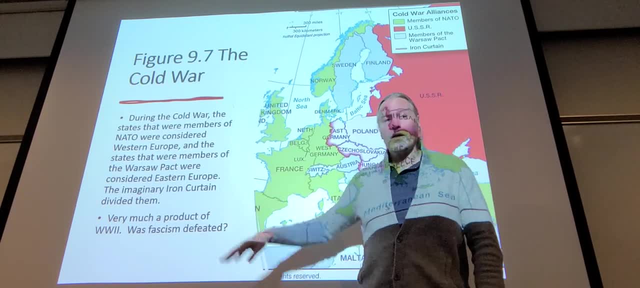 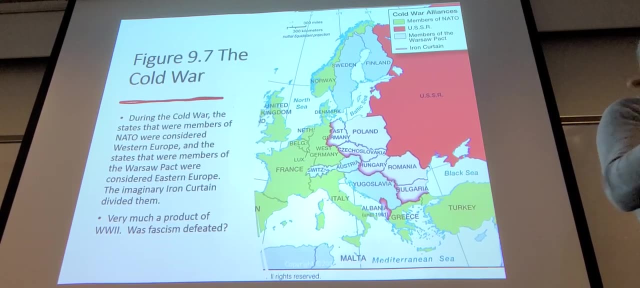 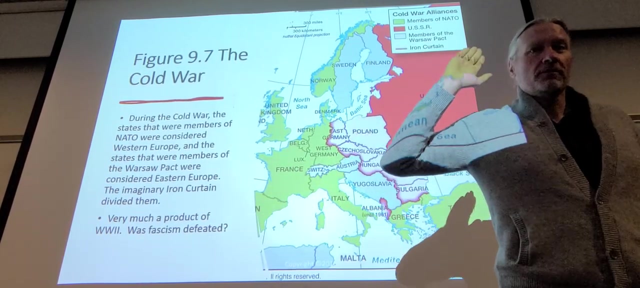 well, that means that you had a police state in these countries. you had um execution and torture of political dissent. you also had, let's talk, what's that? barcelona, that area in the south east, what's that in the north east? so you had the people of north australia, we had the people of the south east. we had the people of the south east. 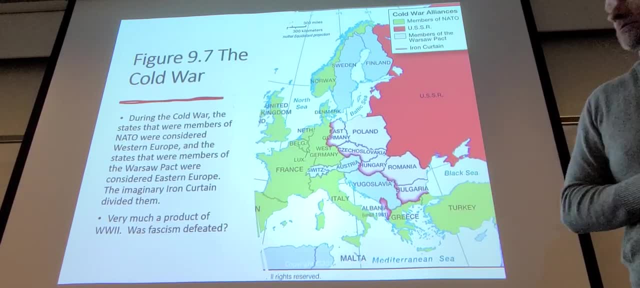 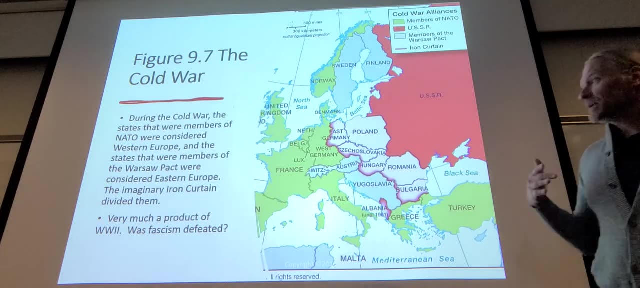 where they fought for their freedom. but they're still fighting for their freedom. Yeah, but Portugal. let's just stick with Portugal for a second, Because they didn't have their decolonial time. after the Second World War, they were still fighting wars in Africa. killing millions of people. for decades, These countries stayed fascist and they stayed empires trying to take resources from the rest of the world by force. It wasn't until the 70s when these countries had internal revolutions. It was interesting because I went to a museum on this recently. 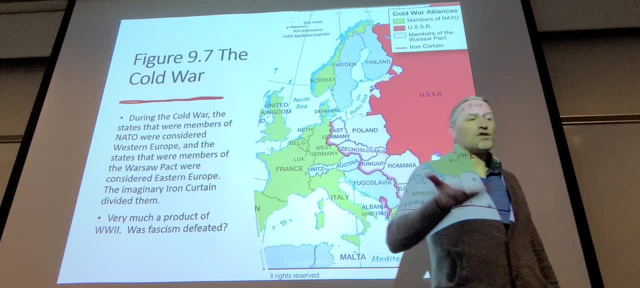 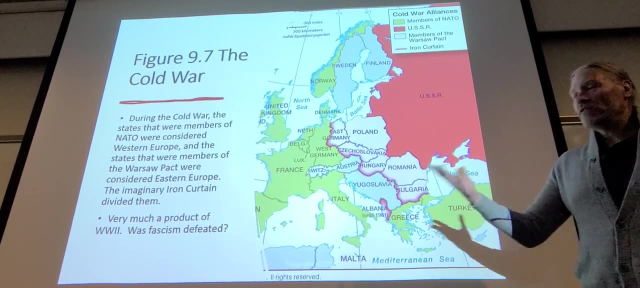 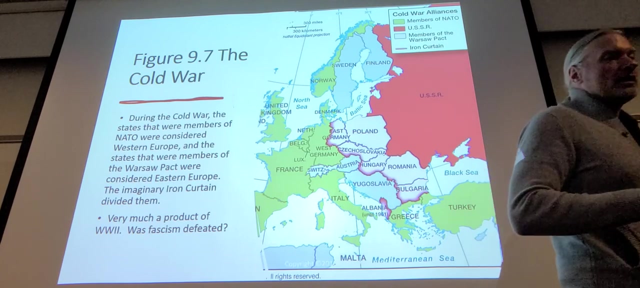 when I was in Portugal and they had an anti-fascist movement that had been going for years and years and years and it wasn't successful until the 70s. And then, when Portugal changed over their political leadership, the country changed overnight. 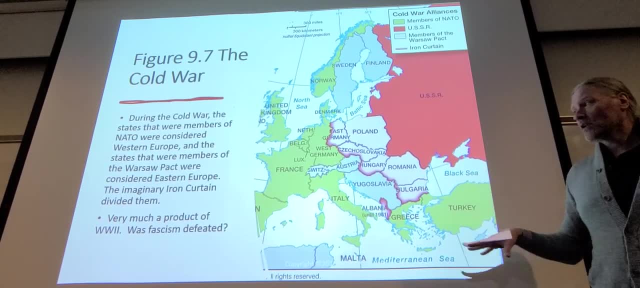 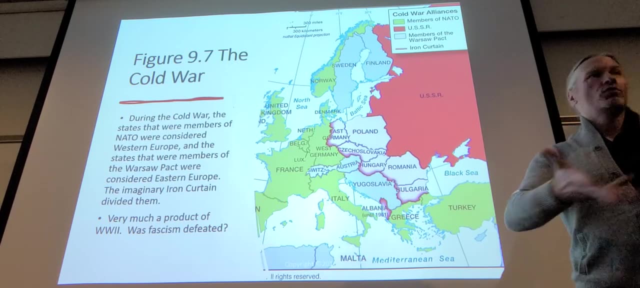 they stopped their wars abroad and they reached out to the countries that had been colonies and they said: anyone who wants to move to Portugal, move to Portugal, you're welcome. So if you go to Portugal, you have lots of Africans. 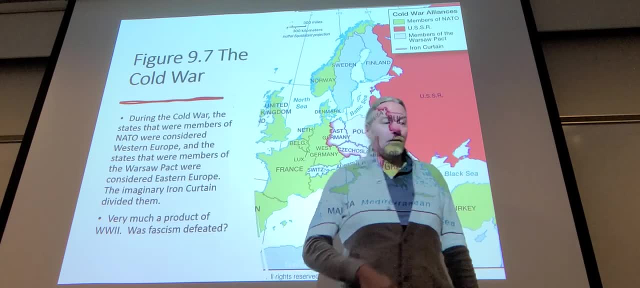 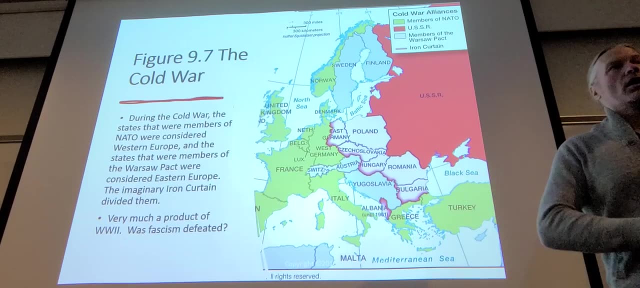 More than a million Africans came to Portugal to live, and their descendants still live there today, So it was a big changeover that happened. when fascist countries fall, It's a different attitude. I guess I would say, Okay, that's a huge tangent. 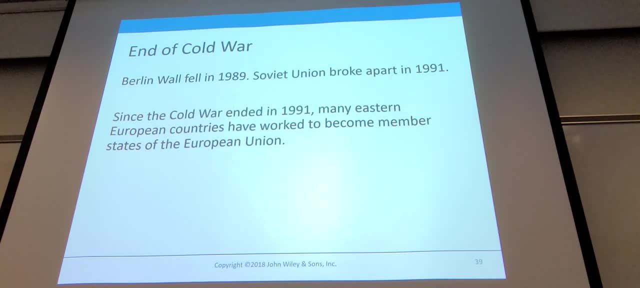 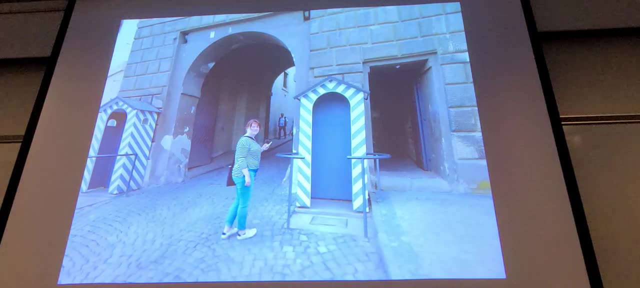 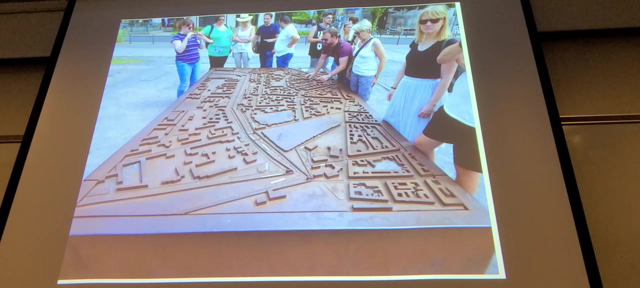 All right, Let's see. Berlin Wall fell. That's when the Warsaw Pact really was no longer a thing. This is the former border. I'm going to show you a little bit of Europe. This is a map. This chapter talks about the Berlin Wall. 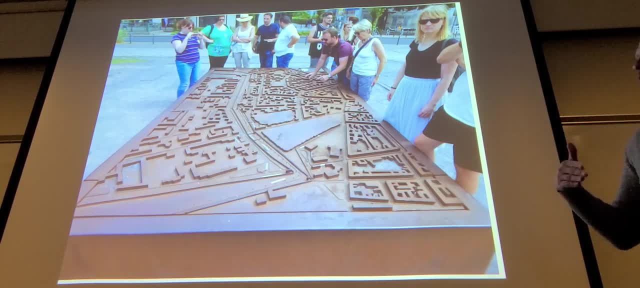 being the big dividing line between the two. This is the big dividing line between the two. This is the big dividing line between East and West. Well, you can go to Berlin, which is a wonderful city these days. Most of the buildings and architecture. 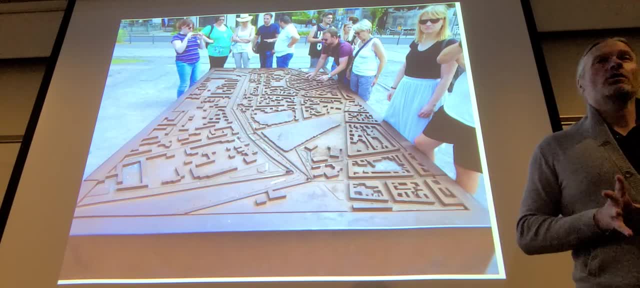 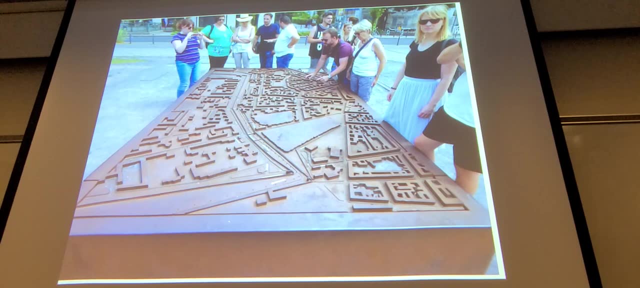 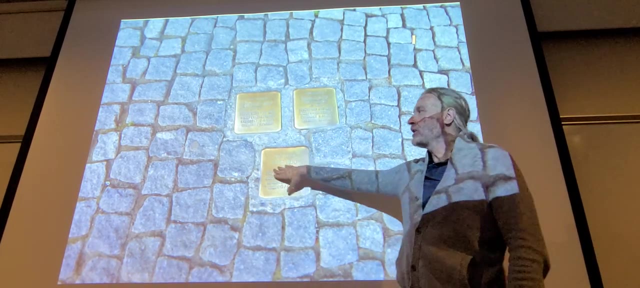 are newer, though, because it was almost completely obliterated during the Second World War. This is just a map of where the wall used to be, and they have walks that you can do, And as you go along these walks, there'll be actual little things on the street. 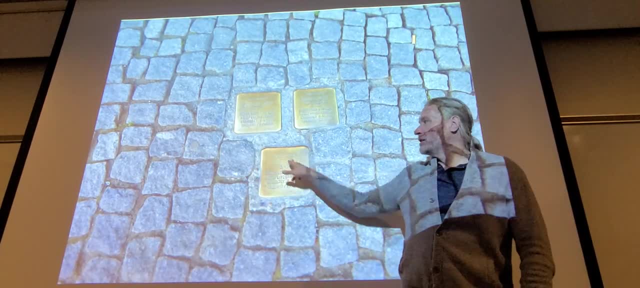 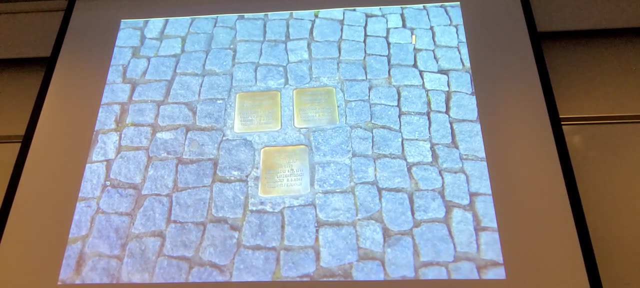 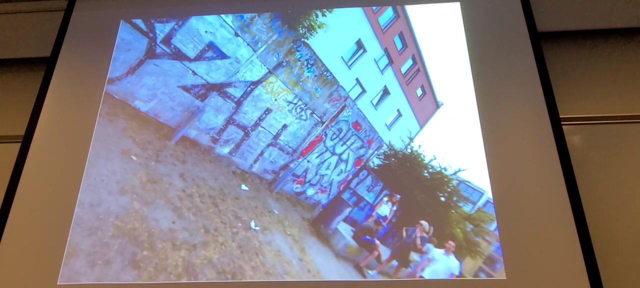 If you're walking around and you notice these things, these will actually be things that list people who were executed during fascism. right, And these are all over the streets. There's places where the wall used to be. Most of the wall's been tore down. 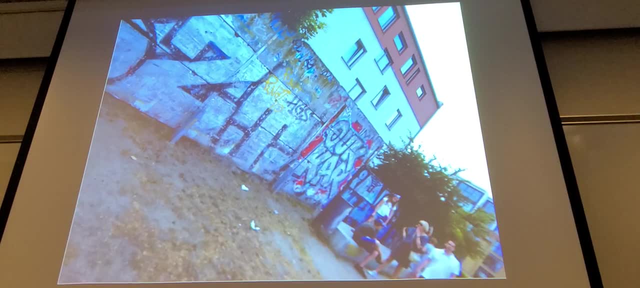 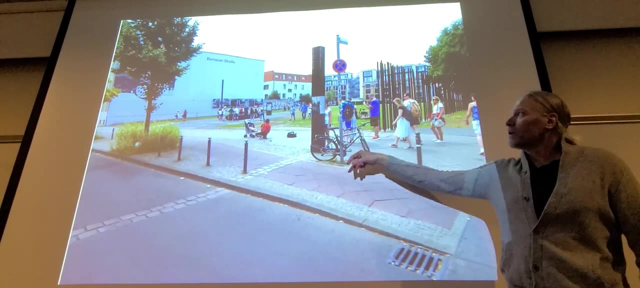 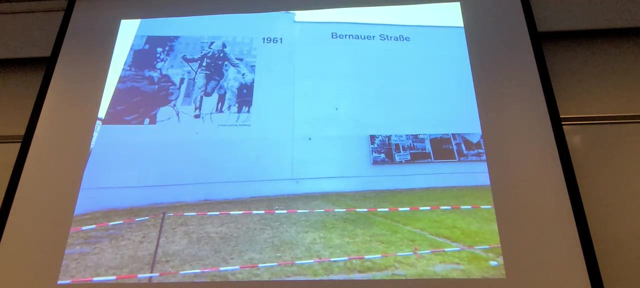 A bunch of the wall. it just kind of looks like this now. It's kind of a lot of graffiti Or they'll have these metal things And, as you can see these pictures on the back, Berlin has a very strong, very strong sense of their own history. 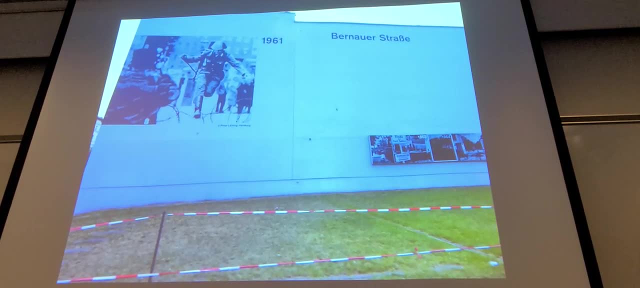 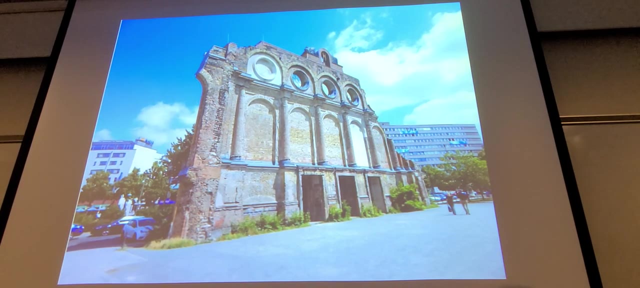 And they'll show you different points along the wall. when people were trying to escape, Different people were shot. Some people escaped. There's, as you go through the city, there'll be slight, little, tiny remnants of giant buildings and structures that used to exist there. 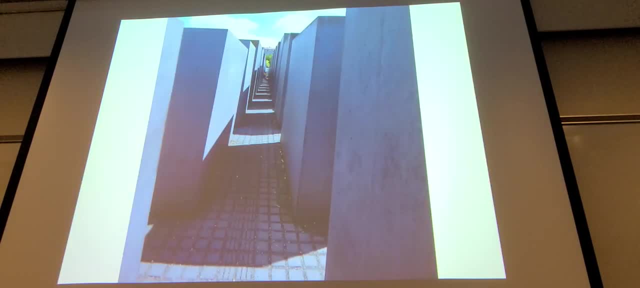 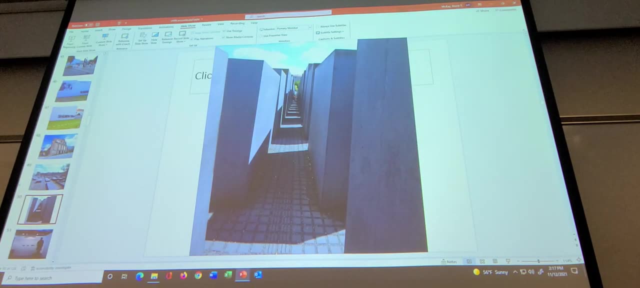 This is a Holocaust memorial, So we're running low on time. So what I'm gonna do, as always, I'm gonna have you guys work on a couple of questions. Oh, let's see here. I think I got them here somewhere.